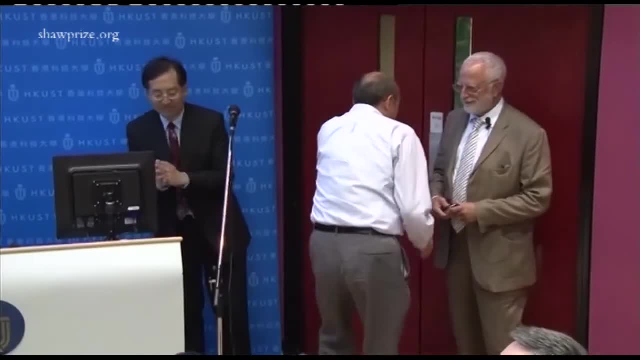 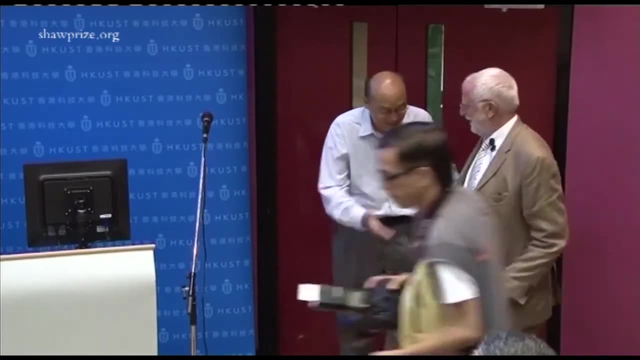 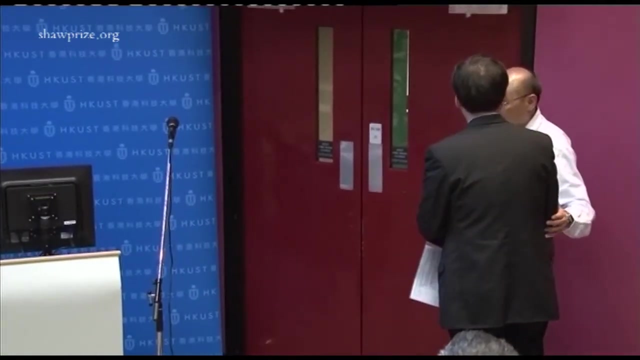 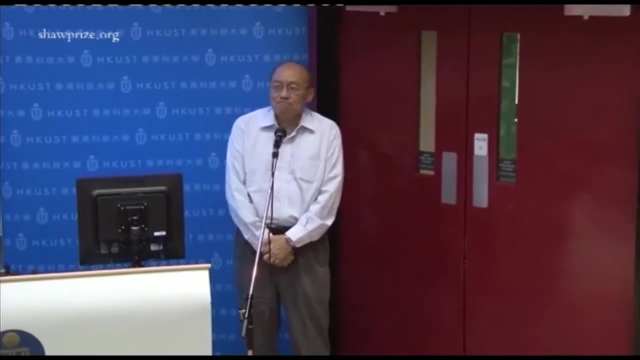 lui. Hi everyone, It's good to be here, Thank you. Thank you, Dr Stan. Mr Broad, Hi everybody, Welcome. This is Anthonyoles Hirschhoff. Anthony, on the line with us in Hong Kong. Hello, good afternoon everyone. 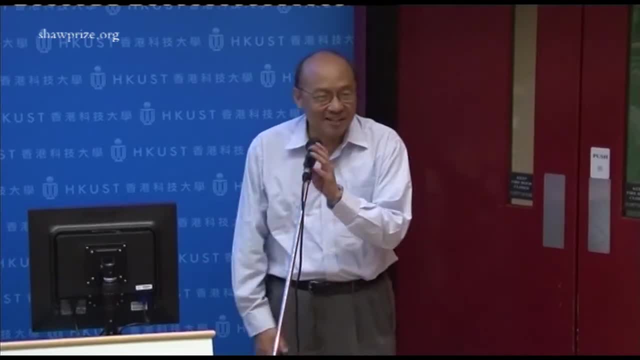 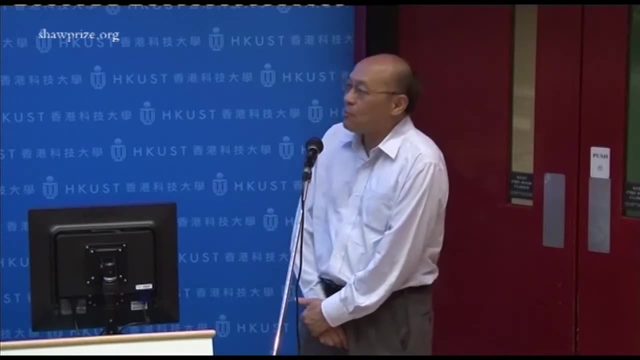 I am Ericisse Sude. and what god date is today for the trabalho mariochi? today, come to introduce our honorary guest today. He's on the way, but I don't know how much longer it will take, So I'm not going to introduce our guest speaker today. 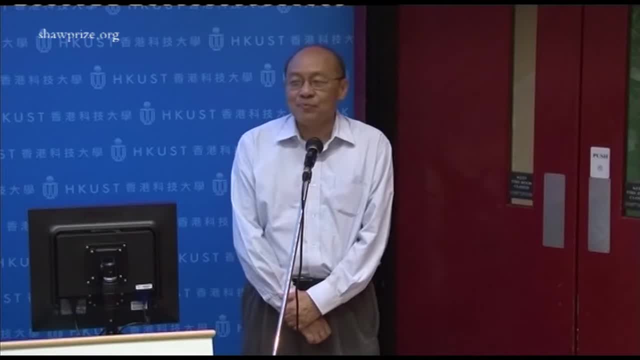 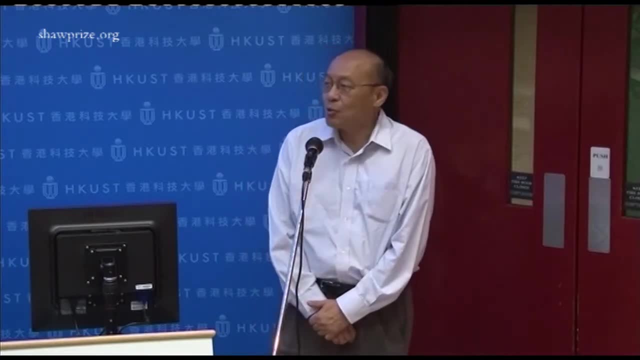 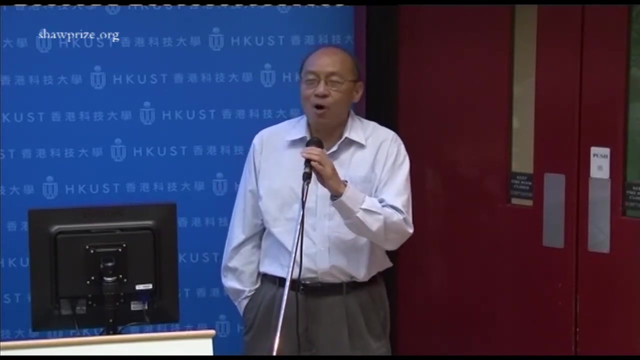 First, because you have seen a very nice introduction already, And second, if Professor Tony Chang can make it, he will give the real introduction. So what I'm going to do is I'm just going to make a couple remarks on the discovery why 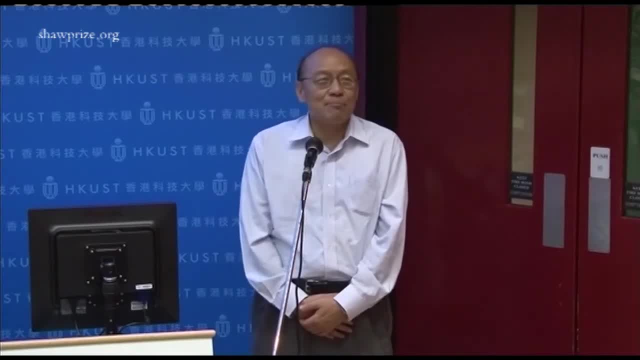 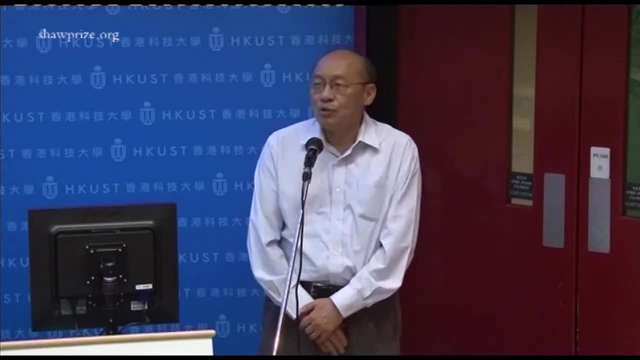 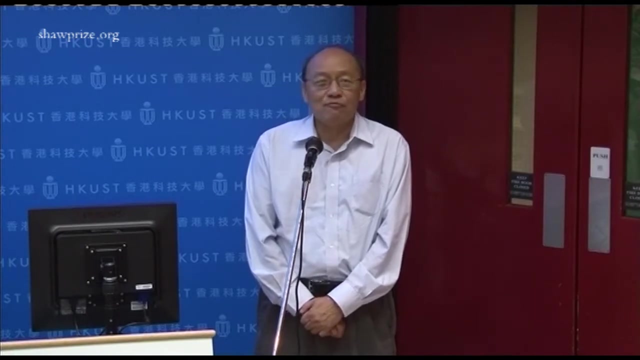 for those of us who is not working in the field, find these gamma ray bursts is such an amazing discovery. As you have seen, and I'm sure Dr Costa will mention again, this actually is a discovery result, one of the few benefits of the Cold War. So it's between US, US and Russia and those days Soviet Union. they want to monitor each other's nuclear test in space. And US launched these Vela satellites to monitor what the Soviet Union will be doing, make sure they're not cheating. 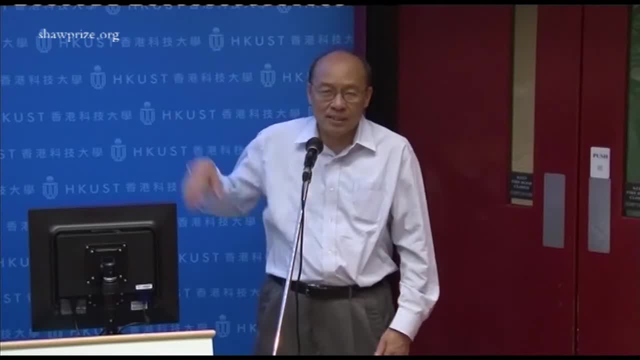 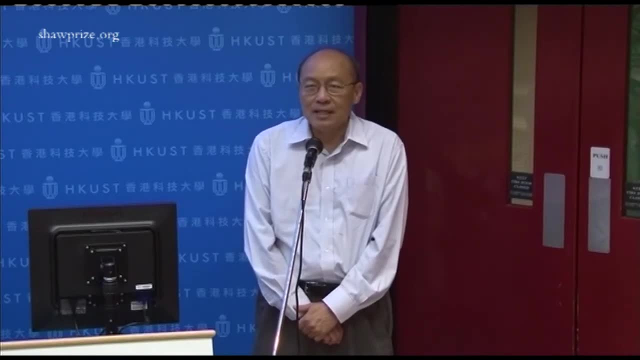 So the satellite is supposed to look on the surface of the Earth, in particular Soviet Union and the Eastern Europe countries, European countries. But every now and then, to make sure things are working or otherwise, they will just look some other directions. 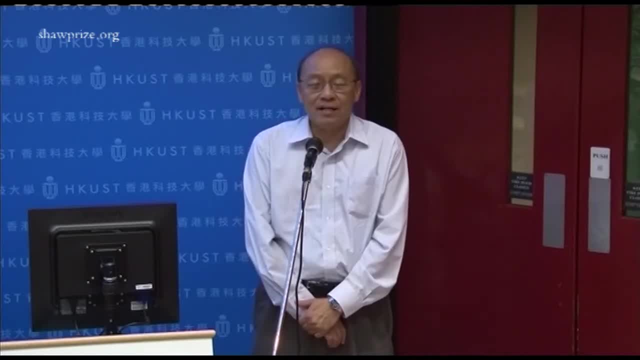 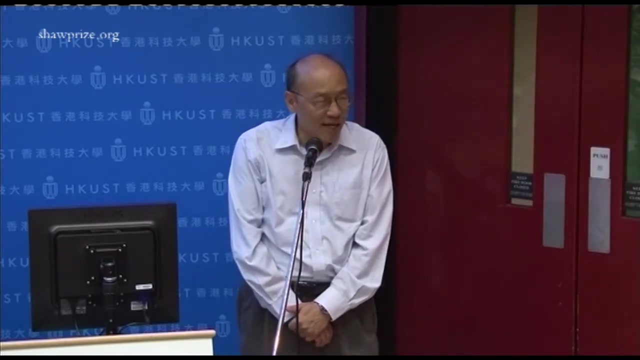 And, surprisingly, they discover some events signal when they look instead of down to the Earth, they look to outer space. They have the data, which they didn't do anything about it, And that was actually analyzed by people in Los Alamos National Lab. 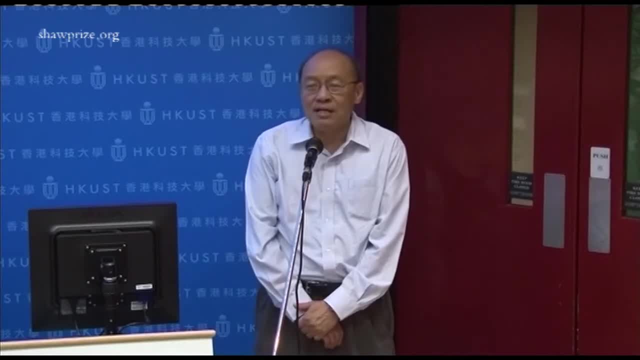 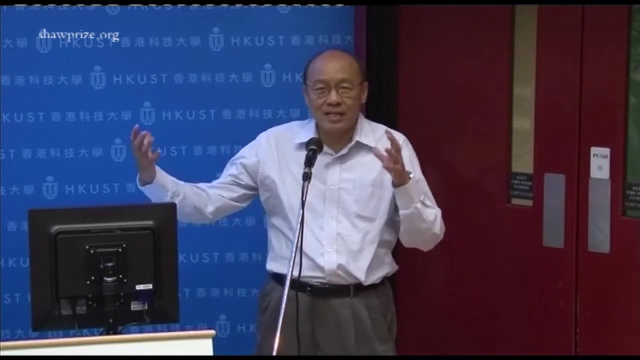 Until they have so much data, they decide to take a look, And, sure enough, by comparison, the timing, the measurements, they discovered the gamma-ray bursts. The big question then is: are the bursts happening within our galaxy, the Milky Way, or it's outer space? 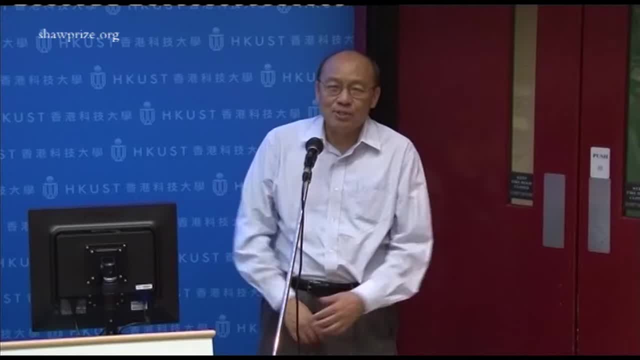 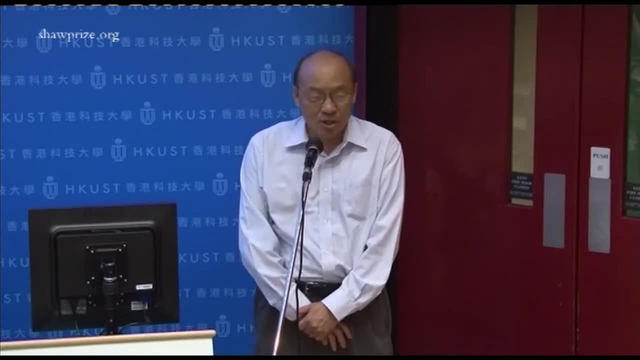 I remember when I'm a student, everybody we talked to said: oh yeah, don't worry, just something happening in our Milky Way And in particular it's outer space. And I remember later on my colleague, Professor Hans Bethe. 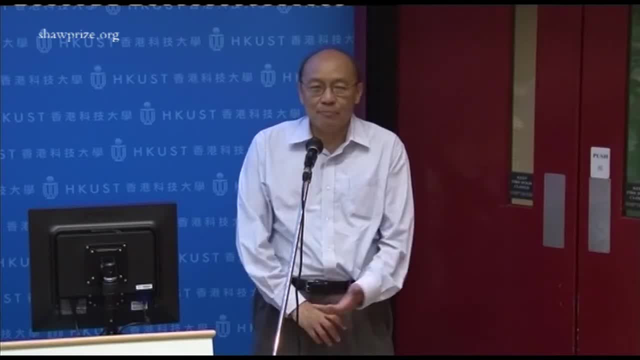 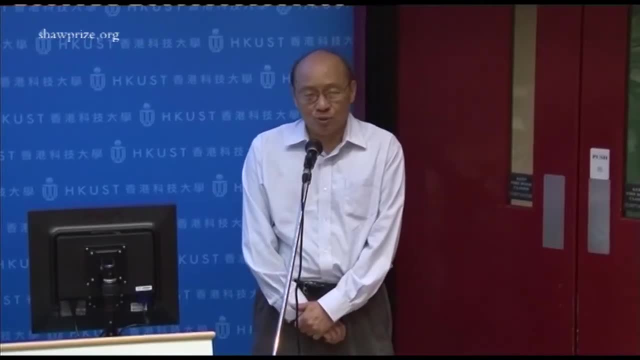 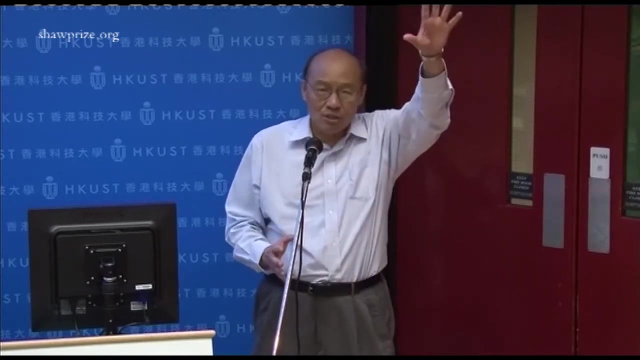 who believed in those days that it must be our Milky Way, because he called me a number called FOE, F-O-E, which is really mean 51-fold. That means the amount of energy produced by these gamma-ray bursts if they are outer, outside galaxy, cosmological. 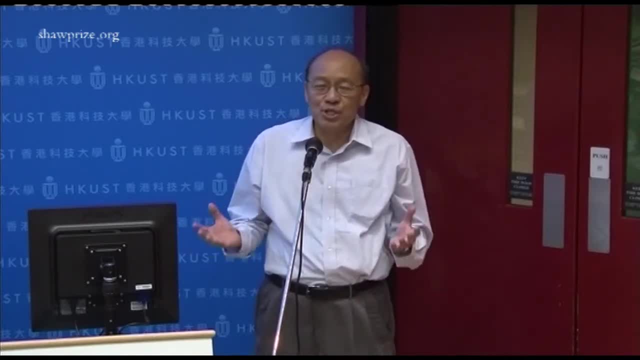 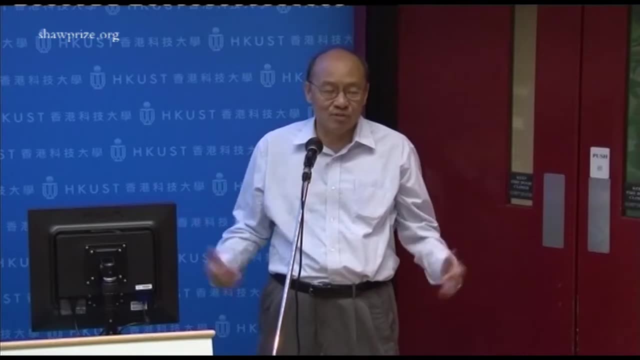 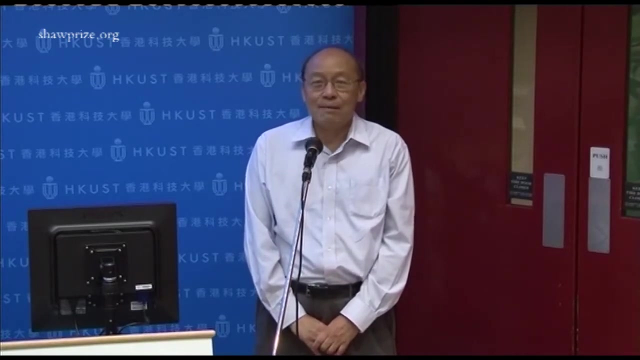 One burst in a matter of seconds will produce so much energy that it will be more than the energy produced by a sun over a period of its lifetime- billions of years. So astronomers, astrophysicists, they all believe it's happening within our local galaxy or Milky Way. 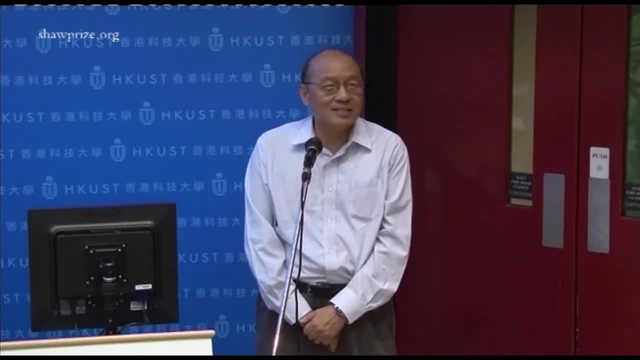 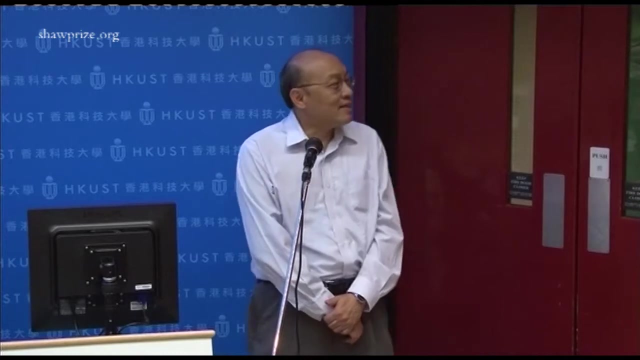 most of them, The few who believe otherwise, have to explain this unbelievable amount of energy being produced. So this is roughly where these things stand, until Dr Fishman and Dr Costa came along. So I think that we may have just a lecture before the introduction by Professor Tony Chan. 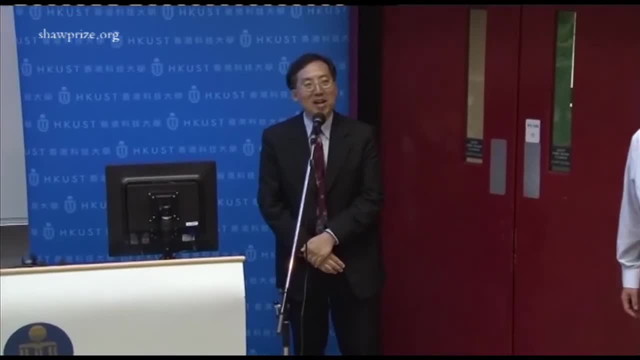 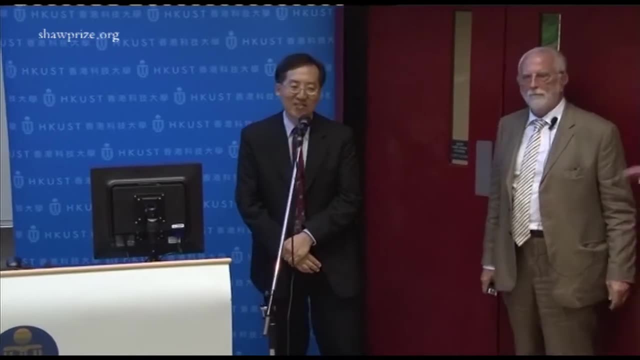 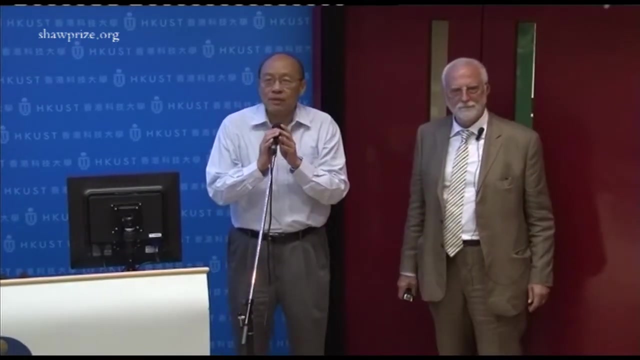 OK, we will now start the short lecture- Astronomy. I would like to add one more point. It will go down in the records as the only short prize lecture in the year 2011.. I should mention one thing is that this lecture will be videotaped. 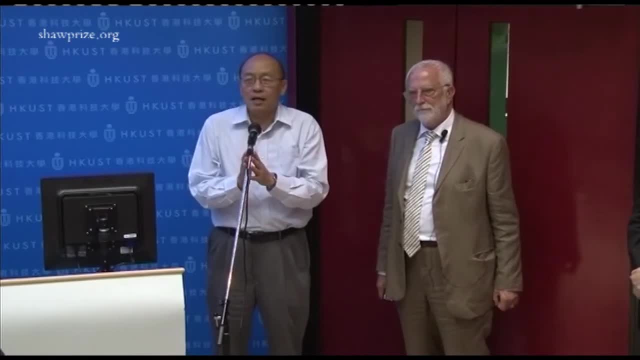 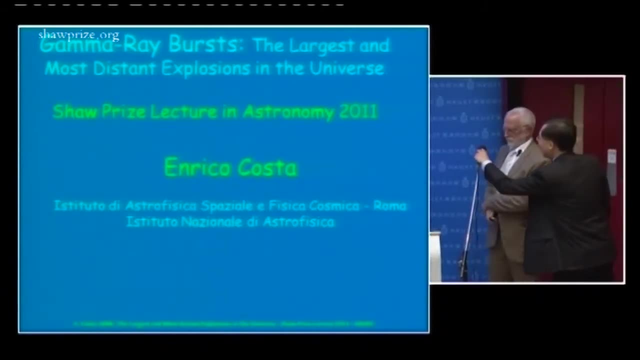 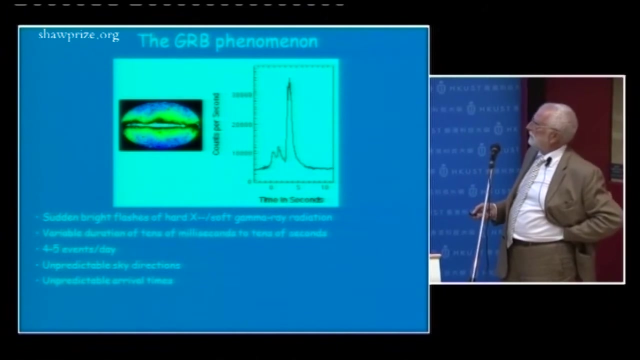 So if your friends who couldn't come, they can go and look at the video. OK, so What gamma bursts are? I'm trying to synthesize in a few slides what Dr Jerry Fishman was supposed to give. There are sudden flashes of hard X-rays or soft gamma rays coming. 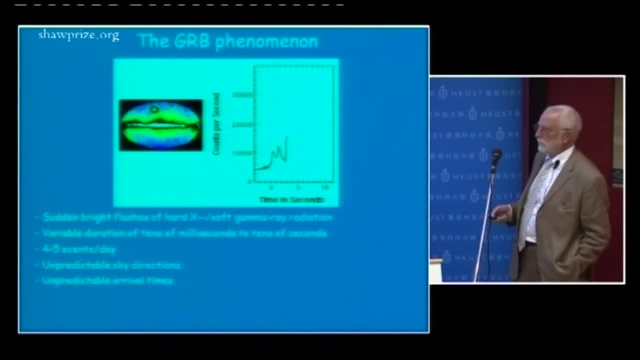 from From different directions of the universe. Then, starting from this statement, it's very difficult to organize these phenomena in some general properties, in the sense that they can be extremely variable in duration, from a few milliseconds to a few minutes, And 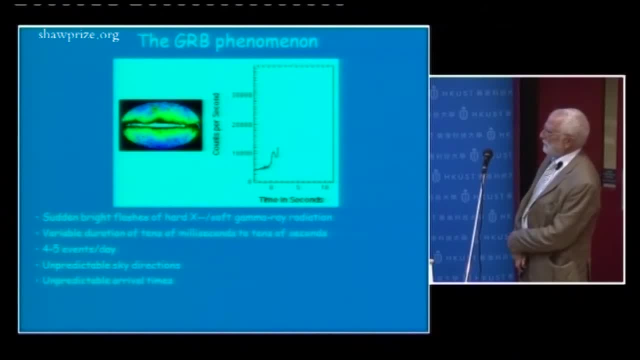 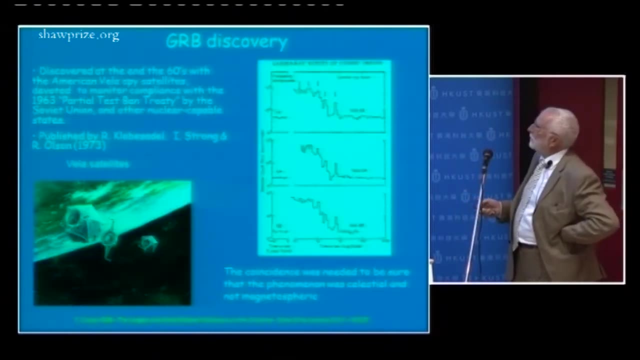 They apparently were never repeating, I mean were never coming from the same direction, And the arrival time was also completely unpredictable. How was this possible, Is that? Well, let's say that the mention about Cold War was very, very specific. 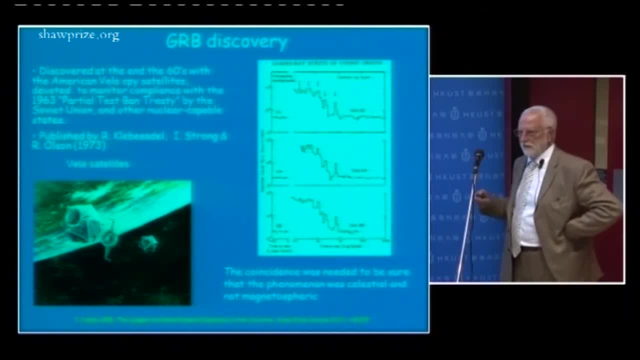 In fact, the astronomy is somehow the domain of large scale. since the velocity of light is limited- or it was until one week ago- We expect typically that everything we observe in the sky is very slow, So to detect something that lasts a few milliseconds you need a special organization of data that. 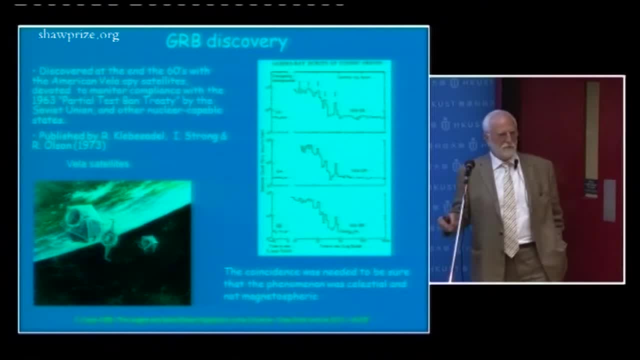 in those times was extremely tough. Nowadays it would be very easy, But in those times it was, And no one would ever build a system with a resolution of one millisecond to do astronomical observation, because no one could expect Pulsar had not been. 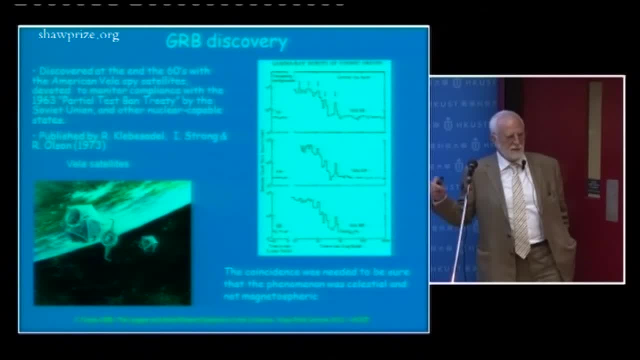 Yet discovered when these satellites were designed. So it was a lucky because, since this was a network of satellites designed to detect the explosions, they could detect some explosion that were not of a human origin, But they were more likely human explosions. One of the point is that when you have a satellite in orbit, you have a lot of particles. 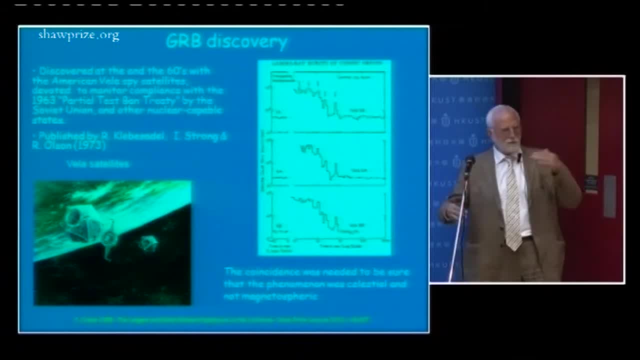 And these particles, depending on the sun, on latitude, are frequently changing, So the satellite may experience an increase of counts with its detector And this is typically will derive from encountering more protons from solar wind. So there should be many tricks to understand that something was coming from gamma rays. 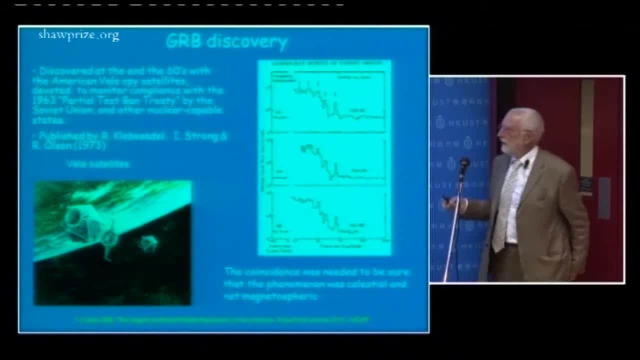 or neutrons arriving from a nuclear explosion and not from an increase of particles due to solar activity. And the satellite was a network. What was required was a coincidence. I mean that two or three satellites should see the same thing and, being far away, this 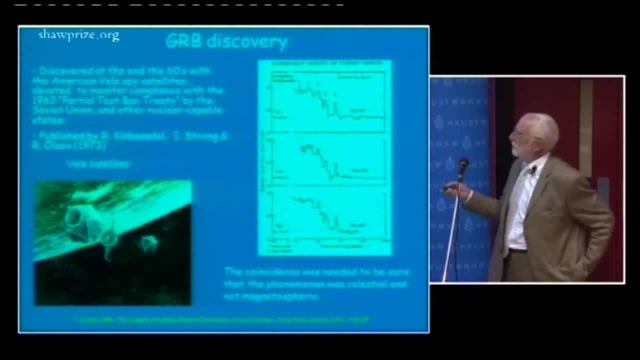 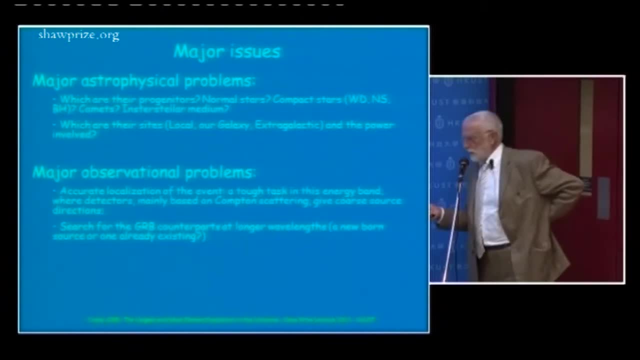 could not be explained in terms of local effects. So which was the problem on, let's say, when it was clear that they were of astrophysical origin, then immediately came out what they are. But it's very difficult to understand what they are if you have no idea at all about the 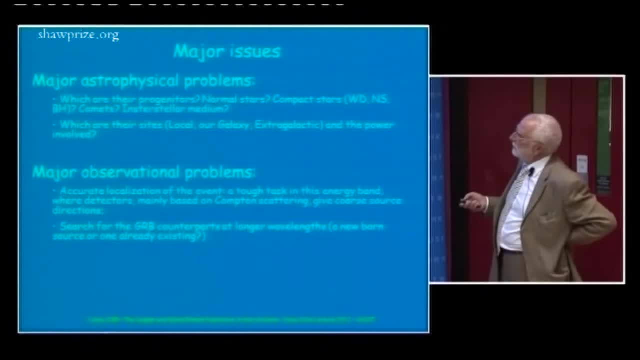 energy involved. One point fundamental is for those who study physics is that the interaction of electromagnetic radiation with matter around 100 kV, 1 MeV, 10 MeV is completely dominated of a Compton effect. Compton effect means that when a photon dies, The photon immediately starts, So it's very difficult to stop gamma radiation. You cannot collimate, but it is also impossible to focus. or maybe somebody is trying nowadays to focus, but it was impossible to focus. So it's extremely difficult to understand which is the direction from which gamma rays. 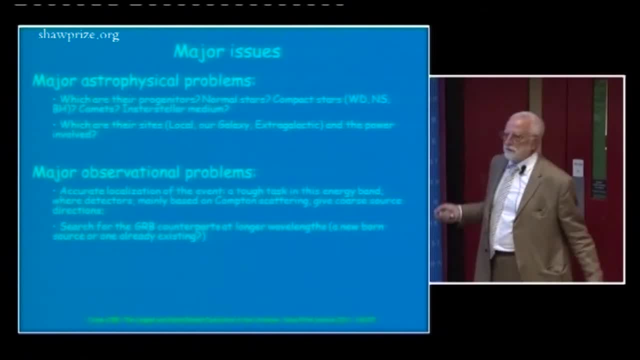 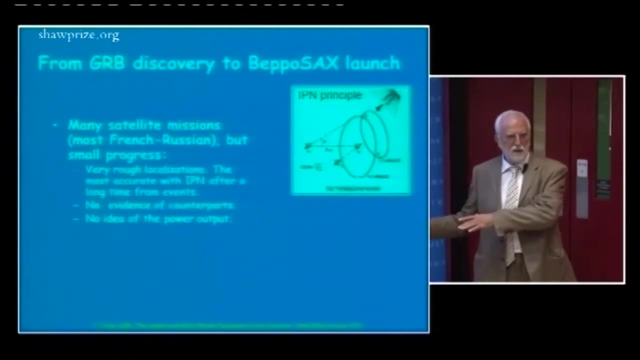 So The hope was to connect this phenomenon with something that could be observed at different wavelengths and eventually, in astronomy, you always end with an optical observation or with a radio observation, because this is why you go at least to one arc, second angular resolution, even more than that, by interferometry, of going outside the space. 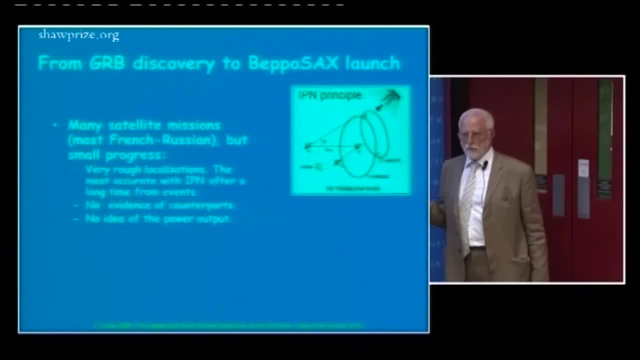 So One way to localize gamma hair before many and let's say for 20 years, the use of a network of satellites and using the delay with which you know if you have two satellites saying one it coming from a certain direction, you have a delay between the scene are recorded. 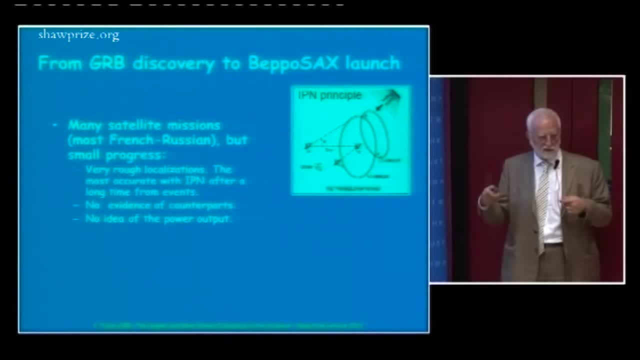 by one satellite and the signal recorded by the other satellite. So one way to do satellite. another way to do satellite is that this idea of lights happening. as you have it, This means that to each delay correspond a cone of directions in the sky. 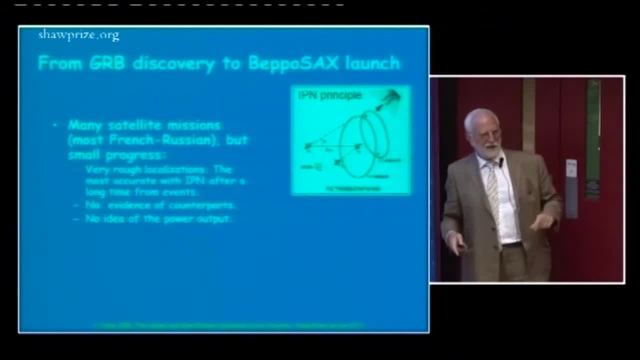 And if you have three satellites, you have three like three coronae projected on the sky and this will cross typically in two points or three. if you have- And this was you can do very well if you have a satellite with an orbit toward Jupiter. 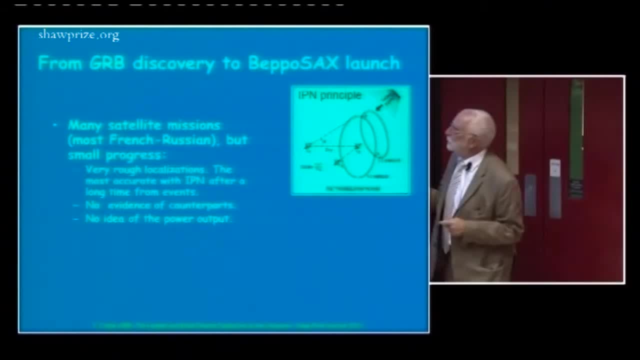 if the level is very long, you can also do good positions. But this in those positions, nothing was found. And this was also because to arrive to manipulate all this data coming from Russia, from in an age that was not internet age, typically could take one year, two years to put together. 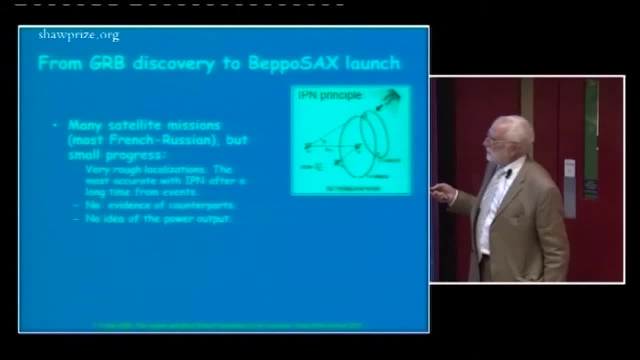 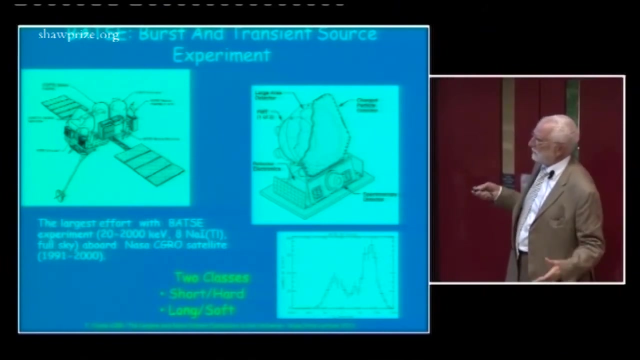 a satellite, All this data, and so there was no evidence of counterparts and the localization was very poor and so there was no reason to assume a certain distance and then a certain localization of other and a certain amount of energy. What the most systematic. 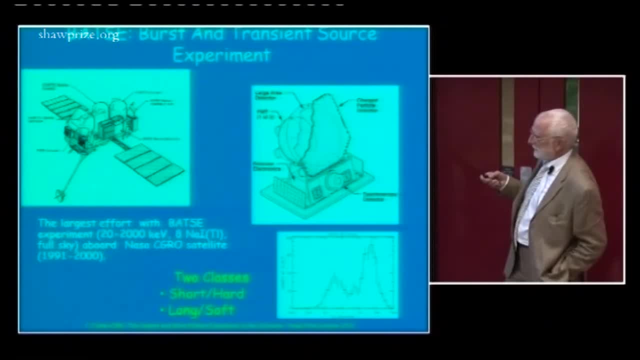 Let's say that some of these satellites were not very well suited to do statistical studies because most of them were not really dedicated to gamma-berth. So when NASA decided to build the huge gamma-ray observatory, very large, very costly satellite- 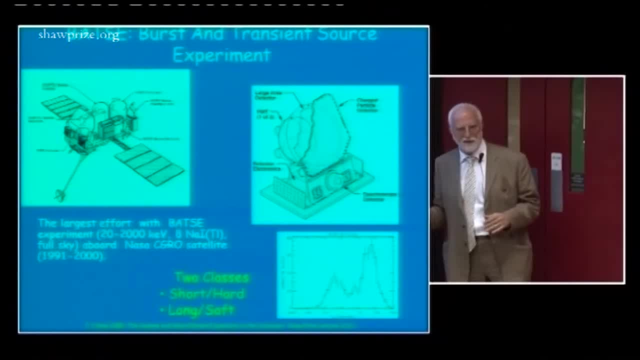 they decided that one of the experiments should be an experimental experiment Dedicated to gamma-berth. So there were eight detectors put in the four, in the eight corners of the satellite and each one would be a very large area detector and they were exposed at 90 degrees, one from 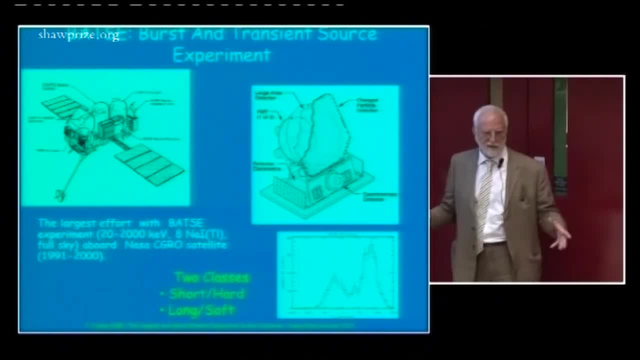 the other, so that they would cover the whole sky and large area to collect many photons. By having in this way A clear vision of the sky, I mean no other instruments in between. they could, for instance, compute how the burst emission was, how the flux was projected on different satellites. 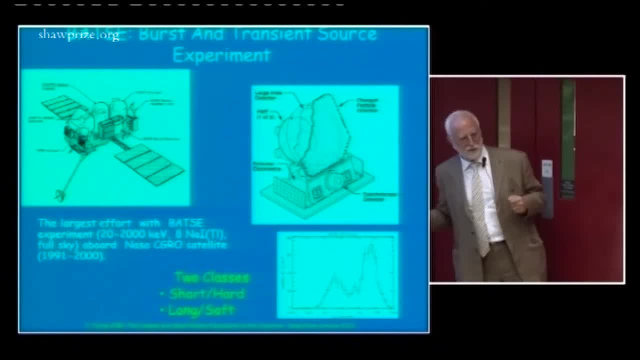 So the first approximation: if the efficiency is one, you can assume that your counts are proportional to the cosine of the angle between, Yeah, Between the normal to the detector and the direction of the bar, And by this you can derive the localization. 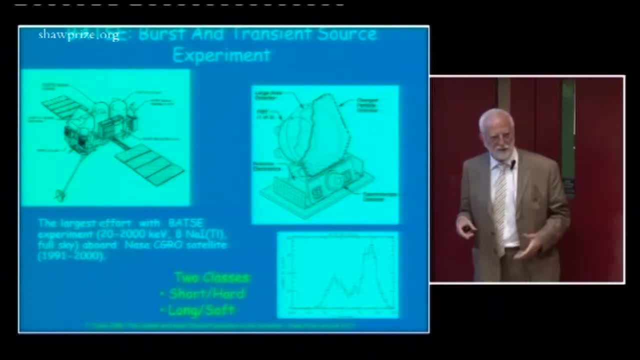 Then if you go back from the geometry to the physics, since this is Compton effect, this is completely different. if you're detector a low energy step efficiency, one at the high energy, the efficiency is very low And this effect is completely different. 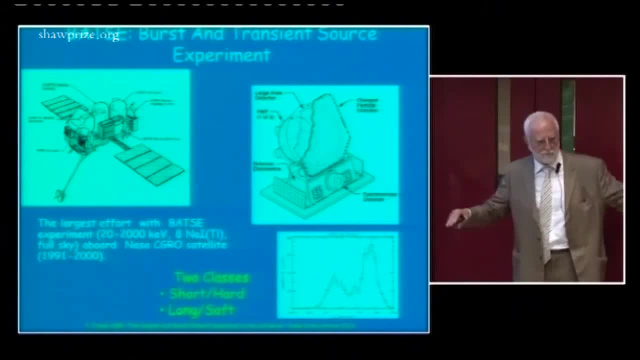 I mean, however you turn your slab, you have always the same counting rate, And then you must use the energy to convert, but the energy is never very well known in a. So let's say that what the Jerry Fishman team did was very important, because they put themselves 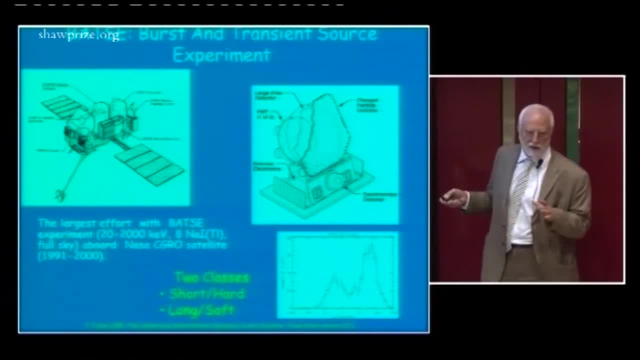 in the position to make, Yeah, A good statistic, a reliable, a robust evaluation of statistical distribution. One of the first things that came out is that there were no possibility to divide the gamma burst in five, six, 10 classes. There were only basically two classes. 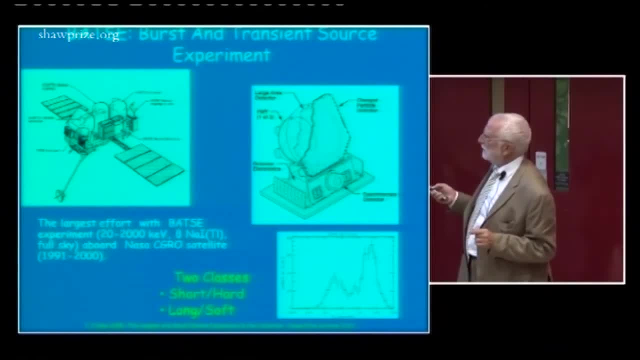 Just taking the duration of gamma burst, you have a long gamma burst, I mean during, From, let's say, two seconds to hundreds of seconds, and short gamma burst from a few milliseconds to a few seconds. They are not completely separated, but if you include also spectrum, the distinction. 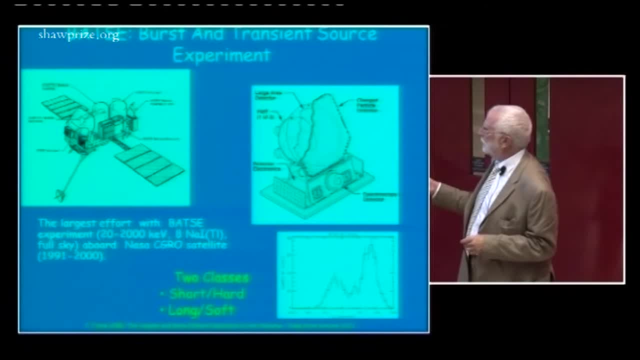 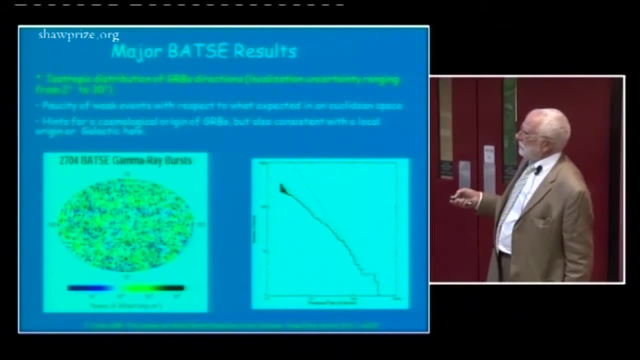 is good, because the shorter are also harder from the point of view of the spectrum. Yeah, The main two results of VASA is: the first is that they are completely isotropic. Second is that there is a paucity of weak burst. I mean that if you make a bigger experiment, 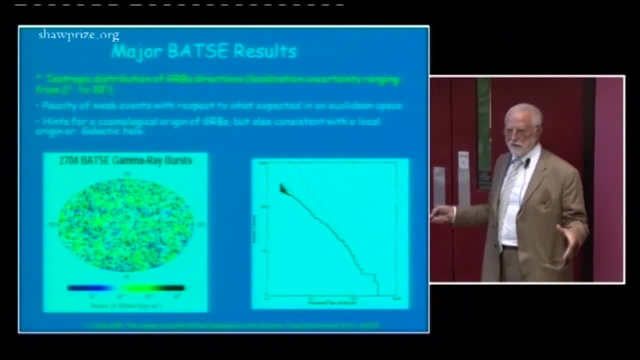 as Dr Fishman did. you increase your sensitivity. you have the capability to detect more and more burst of less, Less, less fluence or flux, and then you expect that the number of bursts you detect in a function of their flux goes up. with this slope, I mean a slope 1.5.. This is what we have. While Bazzi found that there was a shortage of bursts, it was a clear deviation. I mean, it's like if the number of bursts at a certain distance start to be less than expected on the basis of the same density of events at large distance. 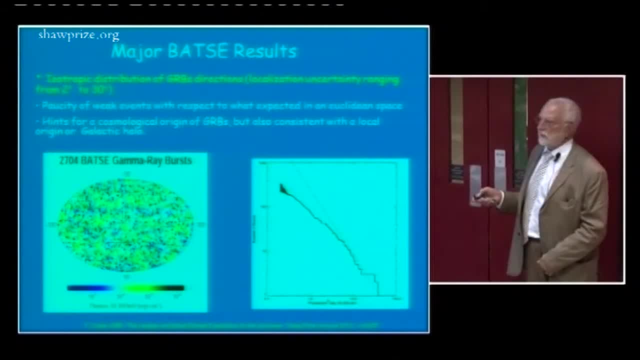 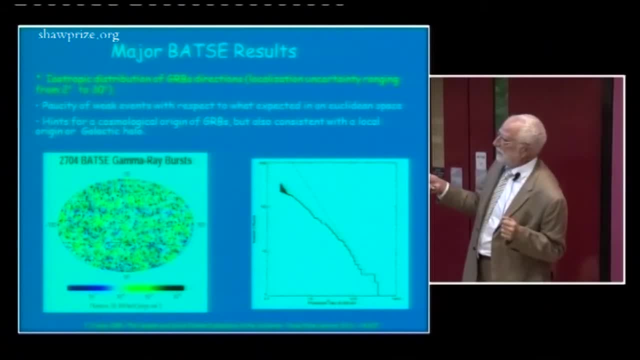 from, like X-ray sources for instance, they would be concentrated around this plane, Even radio pulsars. they are more scattered but still concentrated within the first blast minus 30 degrees. But apparently there was no concentration at all. This would mean that This would mean that there was at least a halo around the galaxy. that means something arriving more or less to the Magellanic clouds, or you know, this was the minimum distance where these bursts could be, But this was still possible, because you know that neutron stars when there is a supernova. explosion and the neutron star is born. if this is in a binary system, it gets a kick. It gets a kick, It gets a kick, And it's a very high velocity. could be launched to a very far direction, so that was not impossible. 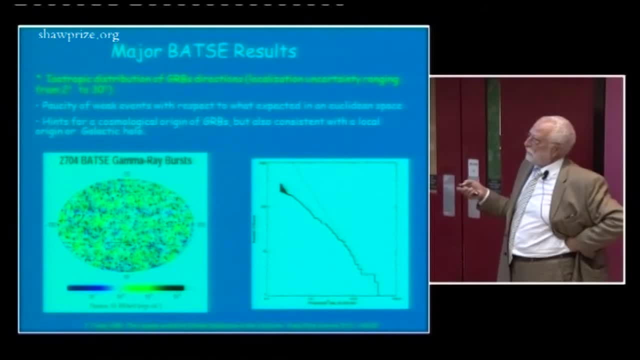 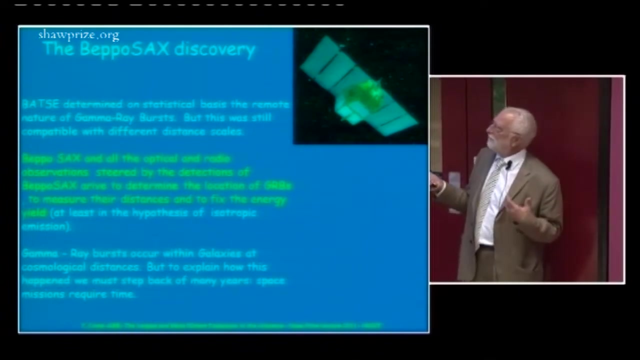 And so I think, the conferences of gamma bursts. still after the BATS results, there was a majority of scientists that were sure that gamma bursts were galactic, and this is because of the Occam Razor that somehow you have the intellectual need. 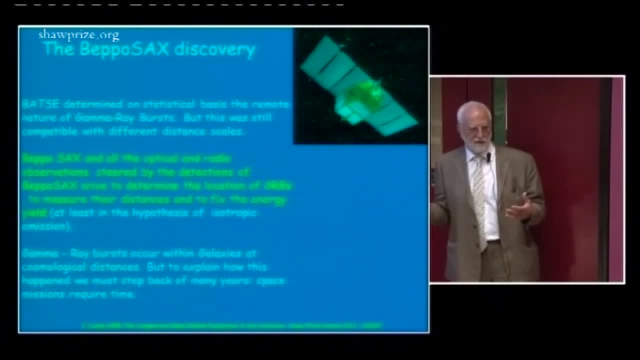 to accept the easiest explanation, Since it's very difficult to assume that you have a phenomenon that can convert a fraction of the mass of the sun into photons in a few seconds. it was much more comfortable to work within something very familiar, an object that do exist, that we know. 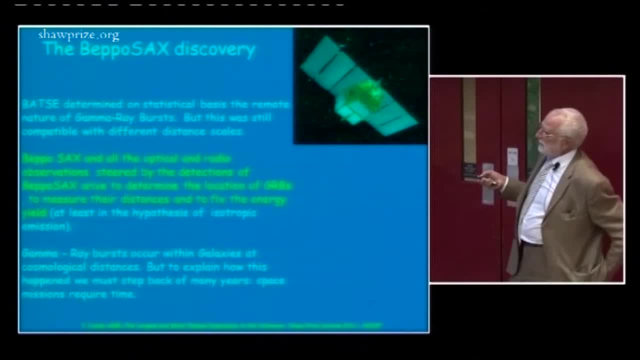 So the second step of this discovery is where we arrive- is that Bazzi gave the statistical evidence that the bursts are, let's say, remote. They come from a distance, But the point was still: are they coming from 50,000 light-years? 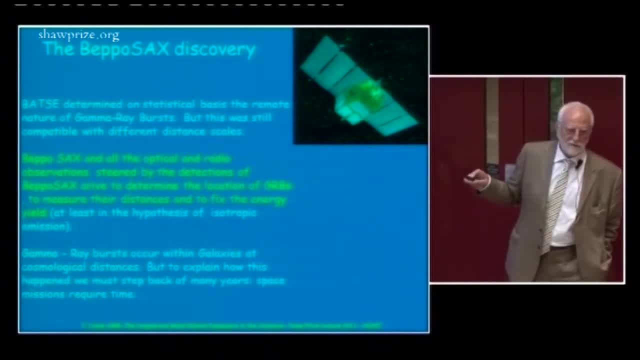 or from 5 billion light-years, which was the real distribution, And what we did with Beposax was something completely orthogonal. I mean, we didn't do any substantial statistics, But we We derived the distance of some specific burst. 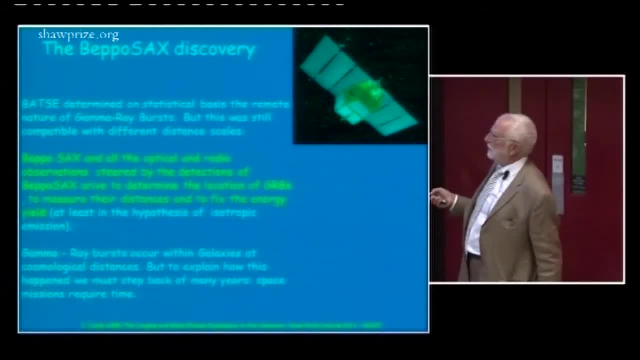 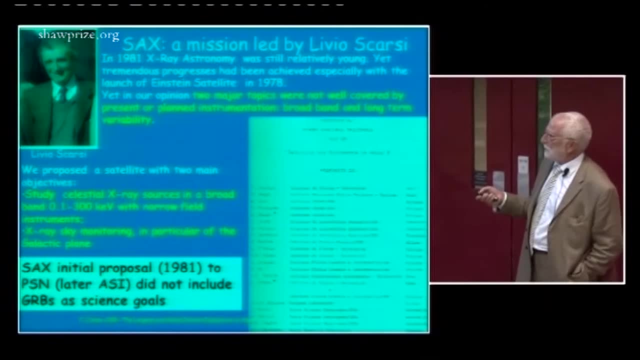 And this, maybe, was the real final solution of this mystery. The story for the people who live that, that's myself- started in 1981, when this is 10 years before Bazzi, of course- when we proposed to the team. 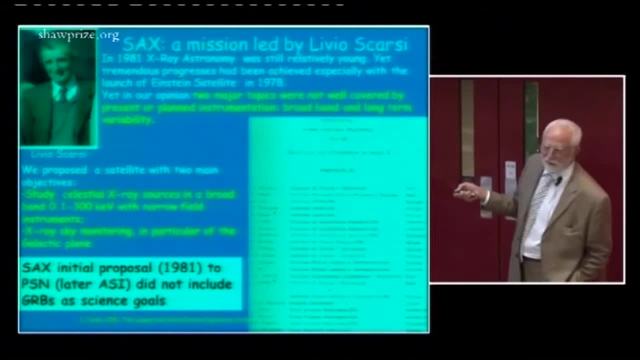 the Italian Space Agency or to the National Research Council- that later became that- to do a satellite of X-ray astronomy. Italy had never done any satellite, of any scientific satellite, And most of our colleagues were considering us mad and were sure that we would never arrive. 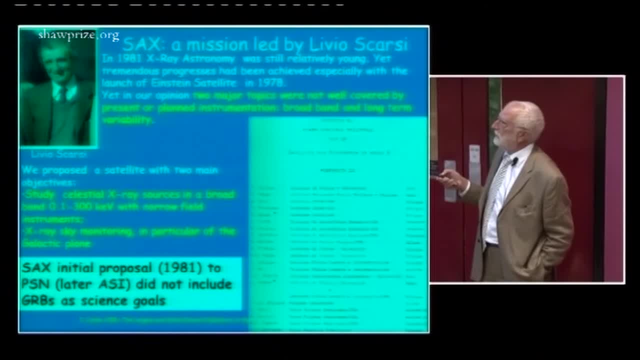 to have a satellite In the space. The leader of this enterprise was Livio Scarsi, a man coming from a studio of showers from gamma, from the cosmic ray showers, but had also recent experience with gamma ray astronomy with Cosby satellite. 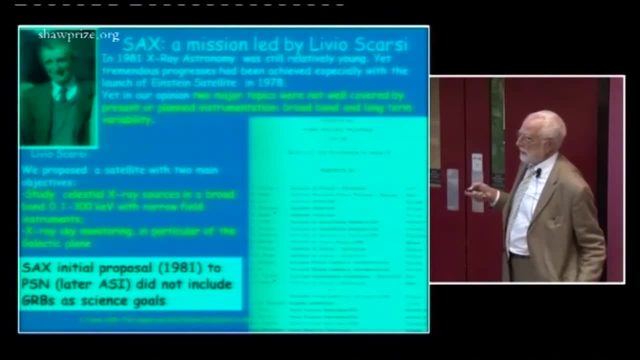 The idea was to have the capability to do studies of X-ray sources on a broadband, because X-ray astronomy had evolved recently. with optics, This means a tremendous increase of sensitivity, but stopping at 3 kilovolts. But we knew from balloons. 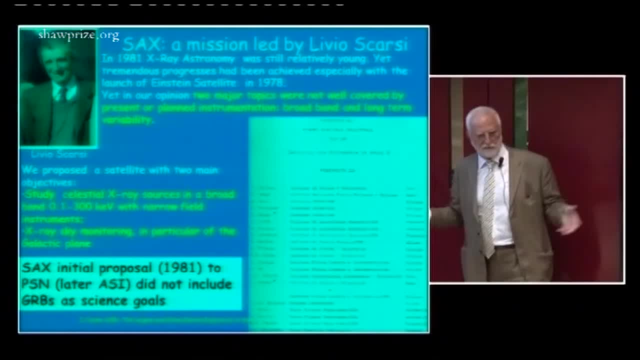 that X-ray source could arrive to 100 kilovolts and there would be a lot of physics in that. So the idea is we should do systematic with the satellite, not with the balloon broadband, and we should have also capability to monitor sources for a long time. 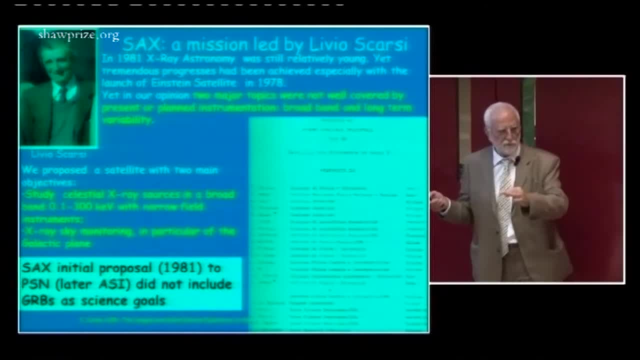 With Einstein, you point the source for 12 hours, for one hour, for one day, for two days, but you cannot monitor for one month for it. So these were the, And originally the satellite had a cluster of narrow field instruments. 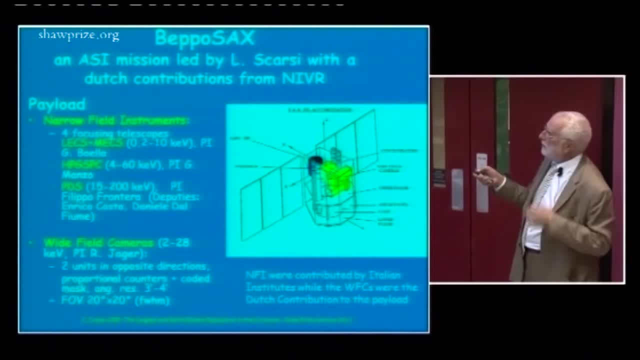 that were all built in Italy and covering different energies: lower energies for telescopes, grazing incidence optics, a four-switch system and a high-pressure gas detector, And then two wide-field cameras that could monitor the sky at 90 degrees from the pointing direction. 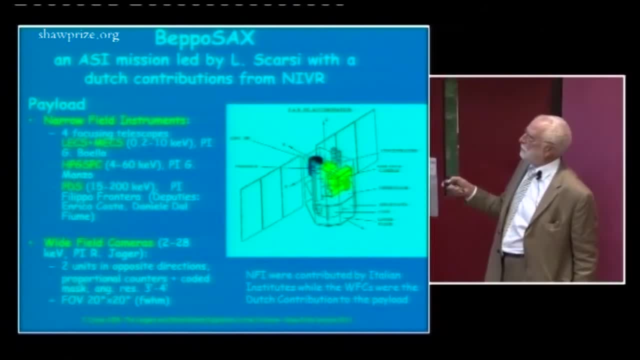 for a long time, I mean while we were doing our observation with narrow field. these wide-field cameras were pointing to regions of sky 20 degrees by 20 degrees, And the wide-field cameras were the contribution of our Dutch colleague. Now what we did. 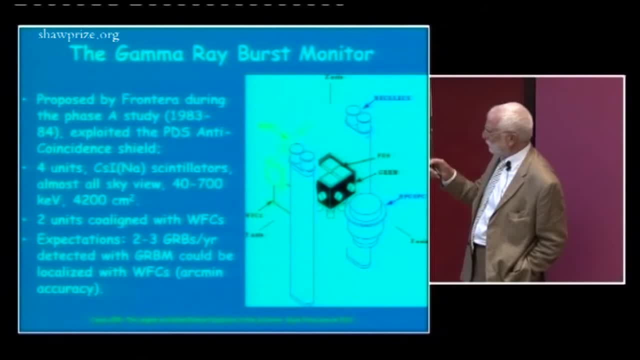 and I had joined the team of the four-switch experiment led by Professor Frontera in Ferrara University, and he proposed to take the shields- four detectors that were used as shields of the four-switch experiment- and by just adding a relatively simple additional electronics. 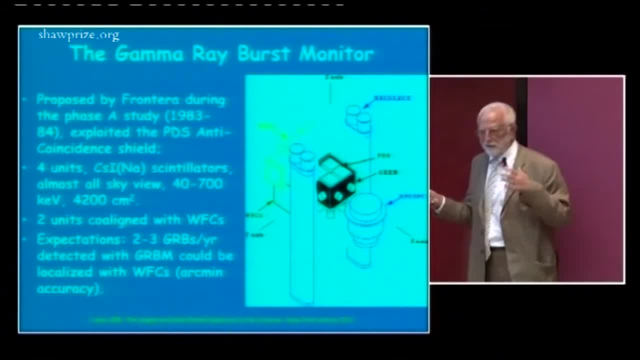 convert them in a gamma burst monitor. I mean an instrument capable to tell that a gamma burst had been detected. The idea was exactly because you saw that Bazzi was outside the satellite. This, our monitor, was in the middle of the satellite. 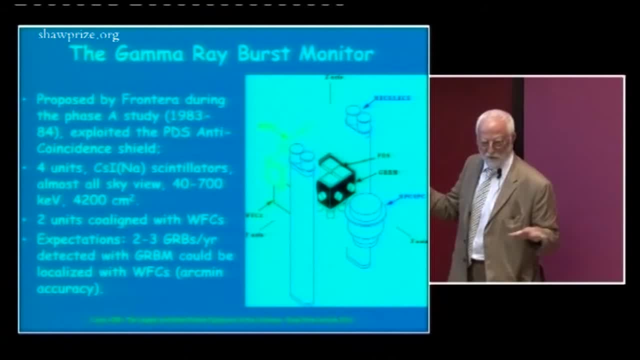 This means that this would never be a good monitor because of the interference of all the others, But it was good because we had X-ray detectors and maybe, maybe, if we knew that a gamma burst had been there, we could hope to see something. 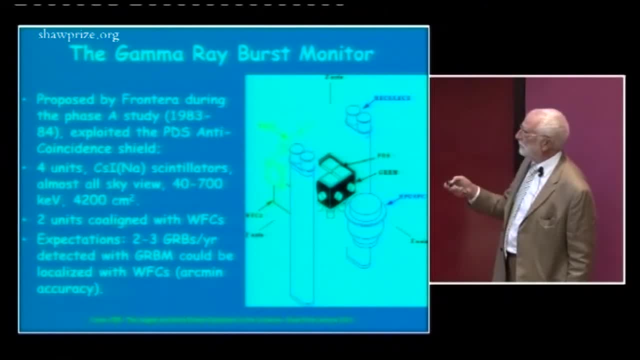 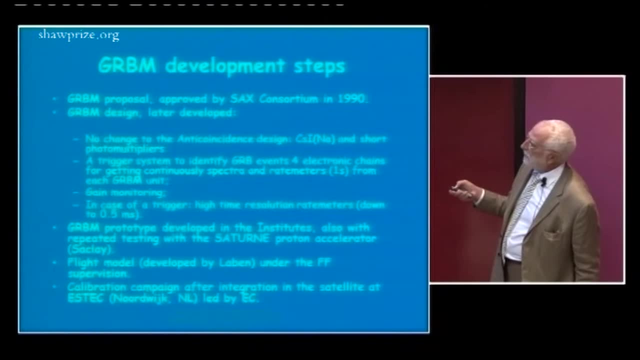 in the X-ray detectors. So we developed this instrument and made various, but mainly it was some additional electronics and a lot of work of testing. simulation Monte Carlo. We arrived to simulate more than 2,000 pieces of matter in Monte Carlo. 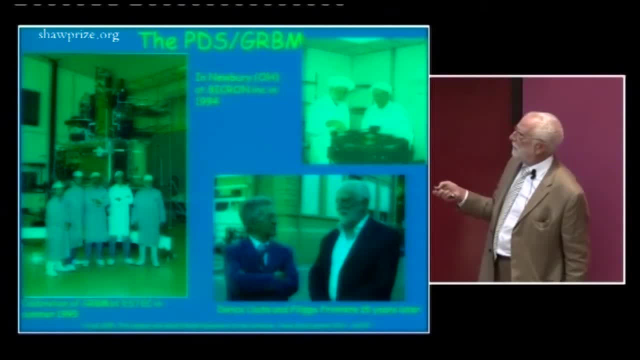 a calibration campaign, And so, after Sachs was approved eventually, it was a lot of work, So this is a piece of our team. This is Professor Fronteiras, the person with whom we did all this work. This is myself in a company. 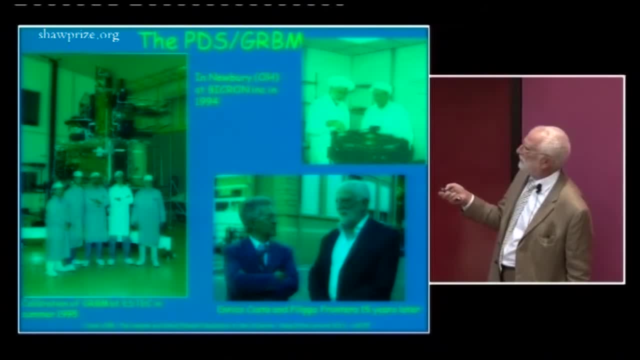 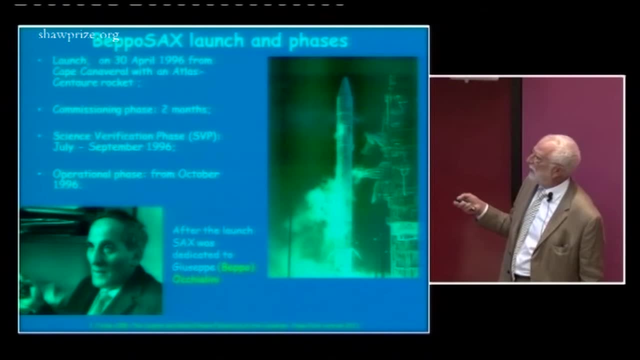 in the USA that provided the detectors And Sachs was launched in 1996, April 30, and after the launch was dedicated to Giuseppe Occhialini, whose nickname was Beppo, who's the man who made the first experiment of antimatter production. 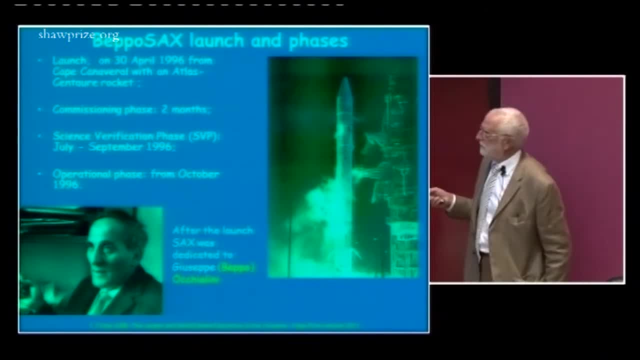 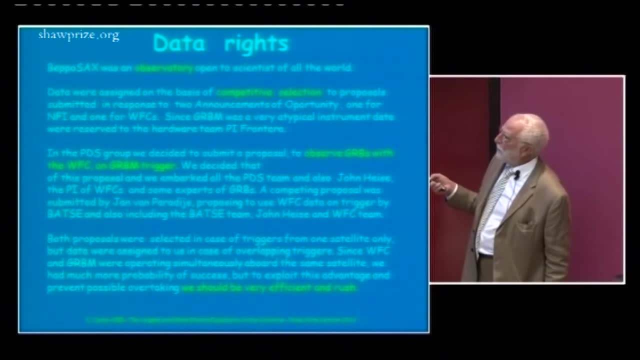 and also discovered the pie meson, And so we named Beppo Sachs. Now what happened is that the data of Beppo Sachs were not the property of the experiment, Maybe data of the gamma burst monitor. they were, because that was not. 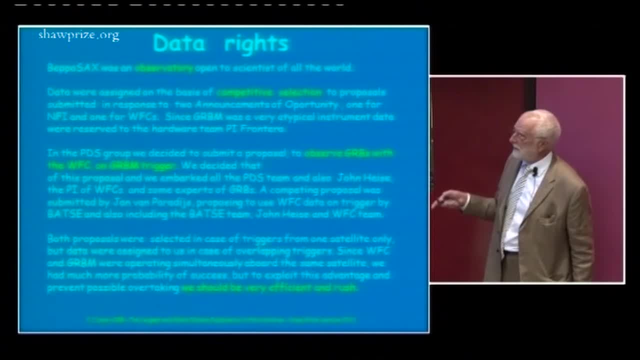 an instrument for an observatory. Data of narrow field instruments and wide field cameras were put in the so-called announcement of opportunity. You say I want to have one month of data of that instrument because I think that with that I can do fundamental. 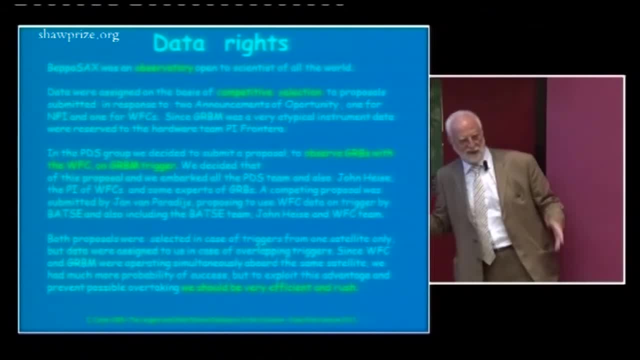 So there is a commission that selected what is thought to be the best proposal, And what we did there was to propose the observation of gamma bursts with the wide field cameras under the gamma burst monitor, And we were approved. Dr Jan Van Paradeis. 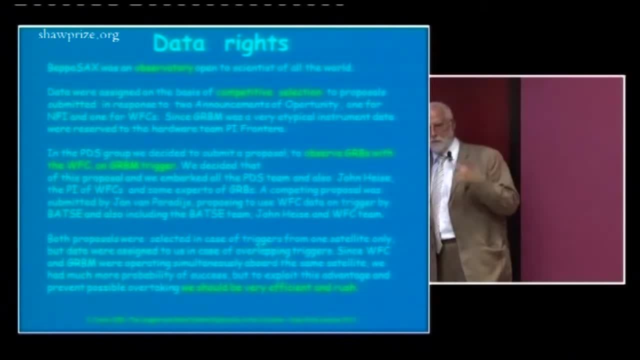 proposed to do the same by using the trigger by BATSE satellite And he was approved with the two. But the point is that since our instrument was on board the same satellite, every time a burst was in wide field camera it was detected by our satellite. 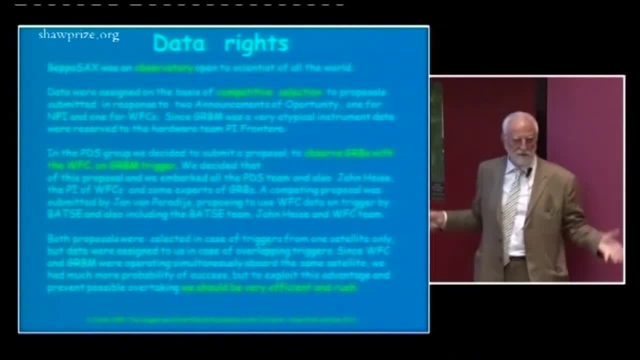 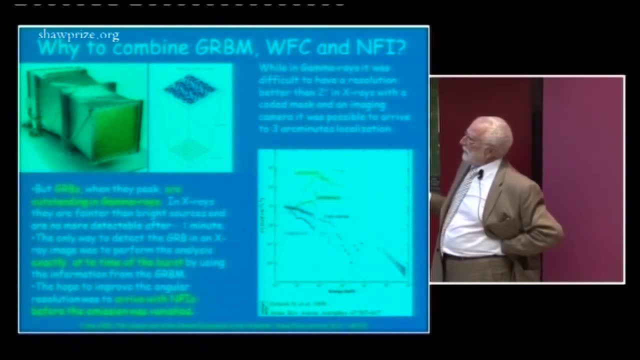 The probability that could be detected by BATSE was much lower. So now somebody say: but you could do everything with the wide field camera without the gamma burst monitor. This is not true at all. Let's see, This is just from a recent review. 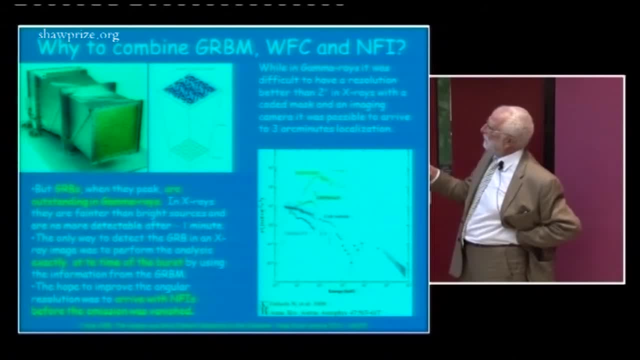 This is a gamma burst, a spectrum of a gamma burst. This is a spectrum of a bright source. The two brightest sources in X-rays, That's Crabbe Nebula and Cygnus X-1.. You see that in gamma rays 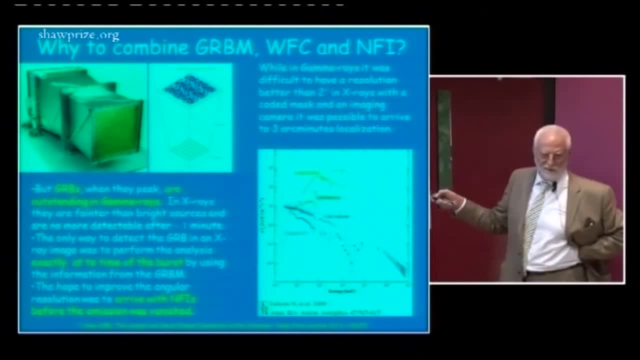 gamma bursts are enormously bright, Brighter than any X-ray sources, 100 times brighter. So there is no question at 100 kV, at 500 kV, that a burst is a burst. There is no chance to confuse with a source. 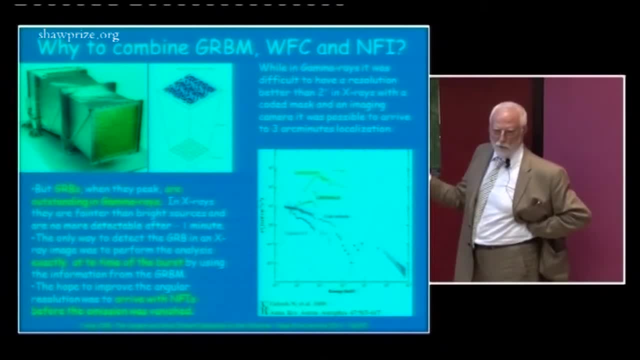 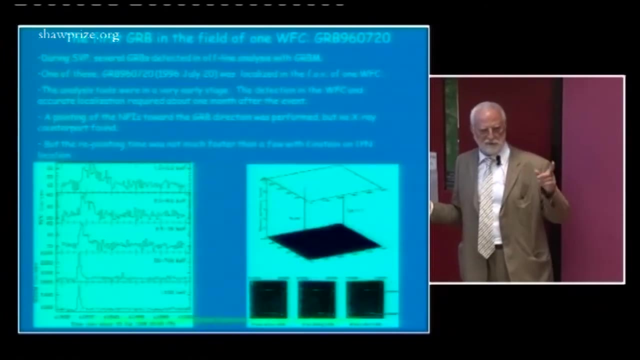 At the X-ray, it's no more true at all. The X-ray source may be brighter than the burst And every time you know that Earth is running around the sky and every source has an Earth set and a down and set every one hour and a half. 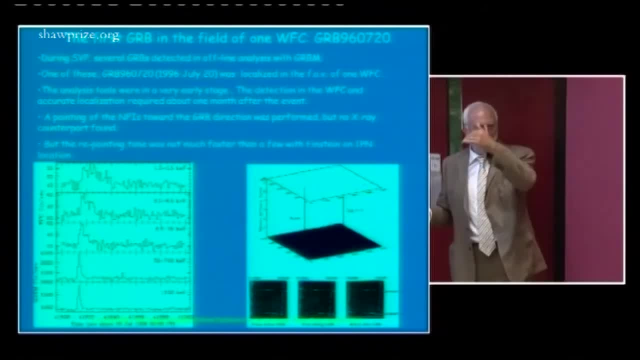 And every time Cygnus X-1 comes out from the Earth, this is a burst if the source. So this was the situation and this was the first burst that we got in the wide field We saw with the gamma burst monitor. 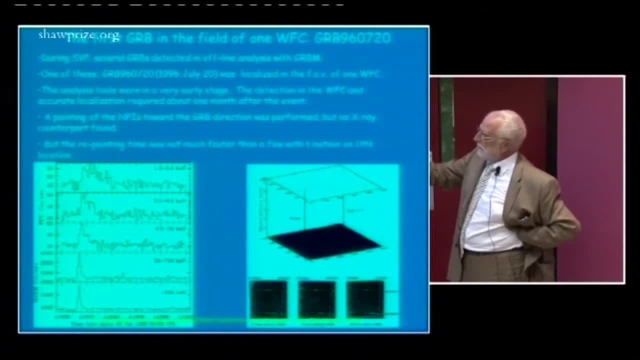 this was a typical gamma burst And then we took data of wide field cameras and took an image at the time of the gamma burst. In this image we found No. first, we found that there was a burst also in the X-rays. 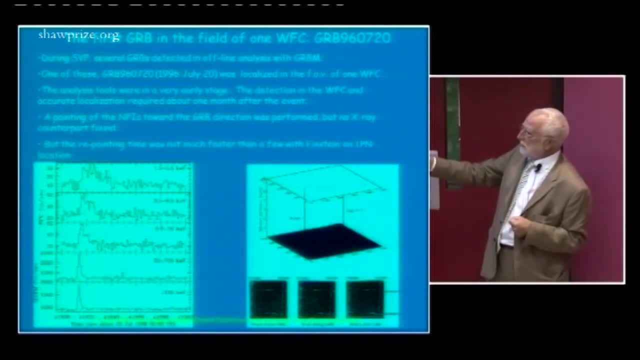 Much more significant statistically. Then, taking the image of X-ray detector, we saw that at the time of the gamma burst monitor there was a source. Before and after there was no source at all. So this X-ray source was associated to the burst. 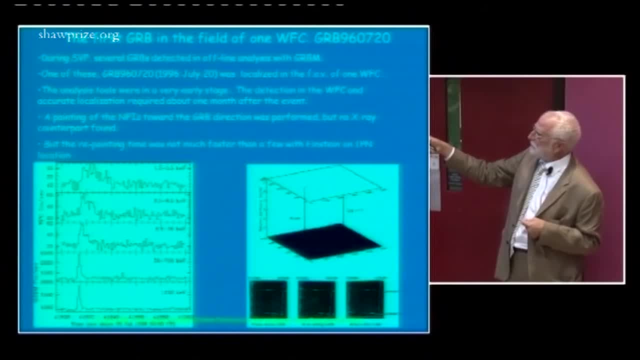 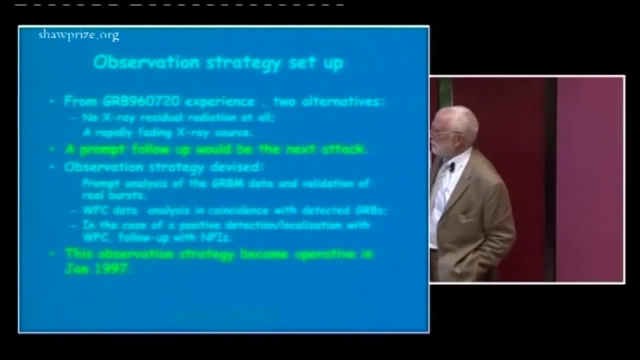 Incidentally, in that first burst there was also Cygnus X-1 in the same field. So we decided that we had the capability to see, to localize gamma bursts in X-rays and we should do that Also because we had been given 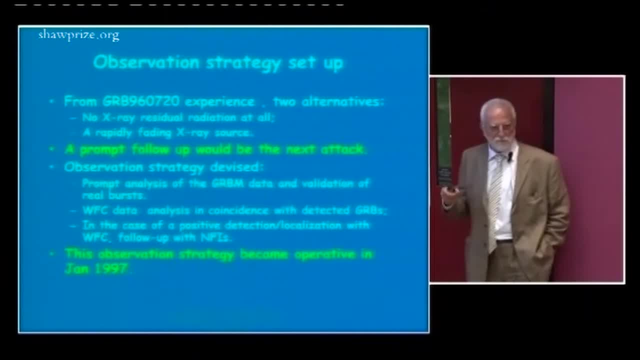 this data under the condition that we would be fast enough and guarantee an efficient use of this data. So we started all the organization of all the satellite systems and organized a process to detect the position of the burst in the fastest possible time and also to turn the satellite. 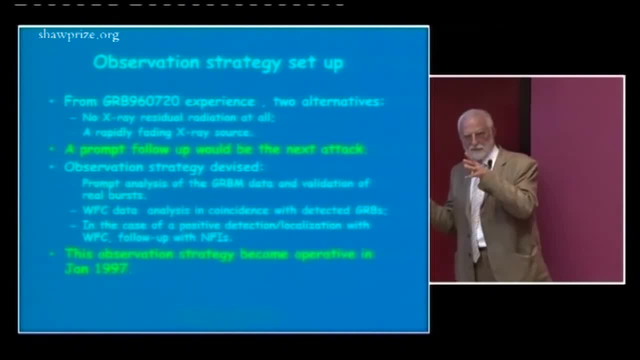 and point the direction of gamma burst with the X-ray telescope. This is because X-rays in the Y field camera, the gamma burst, is visible, but after maybe one minute it disappears. The sensitivity of this instrument is very limited, While with the narrow field instrument. 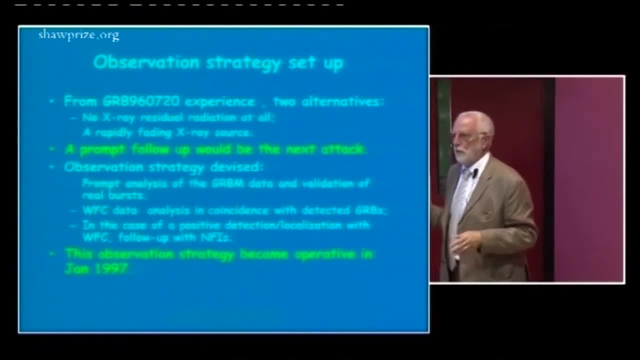 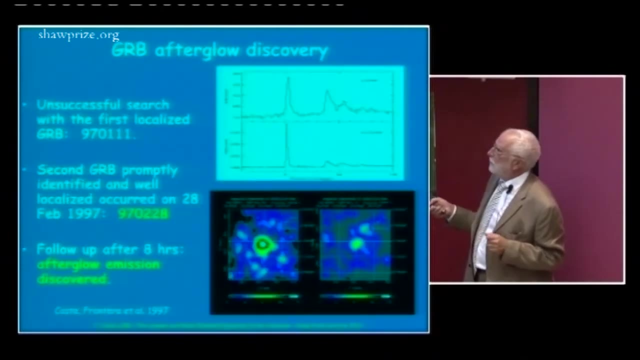 we could have a sensitivity about 1,000 times better than that, or even more than 1,000. So the idea was to point the telescope in the shortest possible time. We had a first chance in January 1st and January 11th. 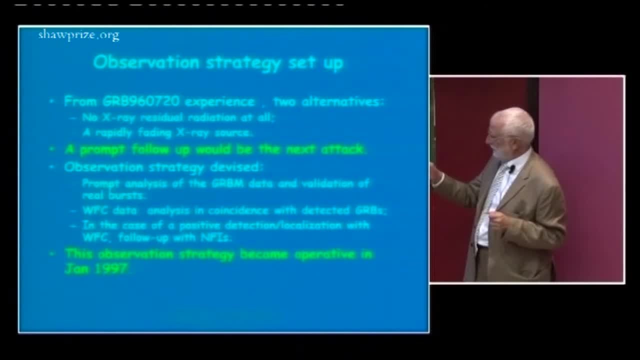 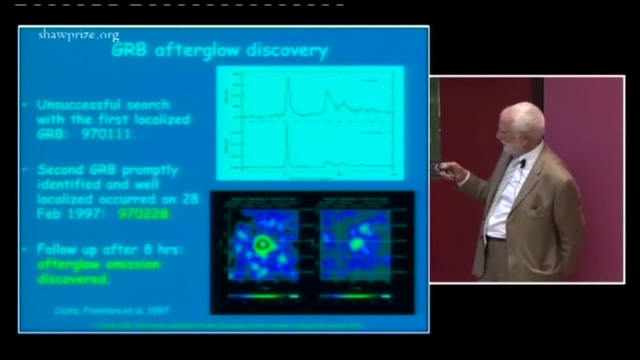 of 1997, but we didn't see anything in the position of the burst. And then on February 28th of 1997, we got a bright burst. We had also a signal in the Y field cameras By accumulating that. 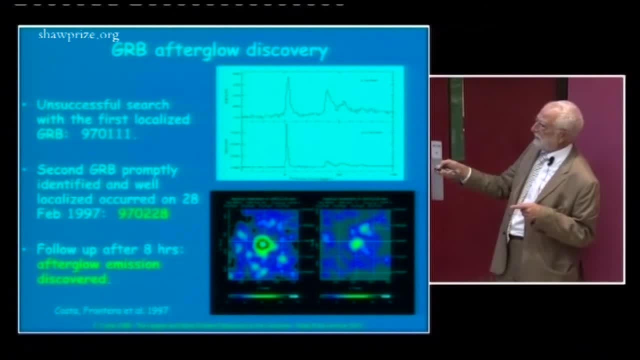 we derived the location of the burst. We pointed, the telescopes and our organization had been shrinked down to arrive to only eight hours from when the burst had occurred in the sky. We found a relatively bright source in that position, The probability to have such a bright source. 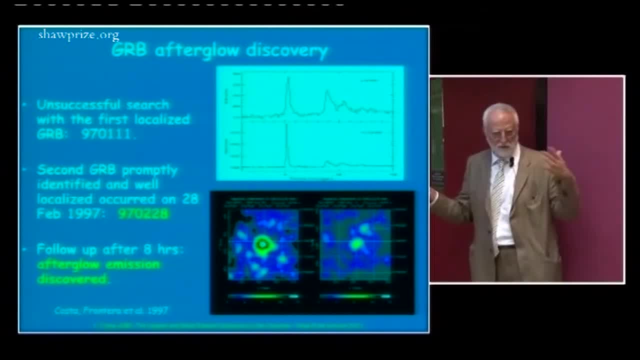 by pointing a chance position of the sky was less than 1,000.. And pointing again: this is February 28th, this is March 3.. We found that the source had a factor of 20.. So putting these points in a graph: 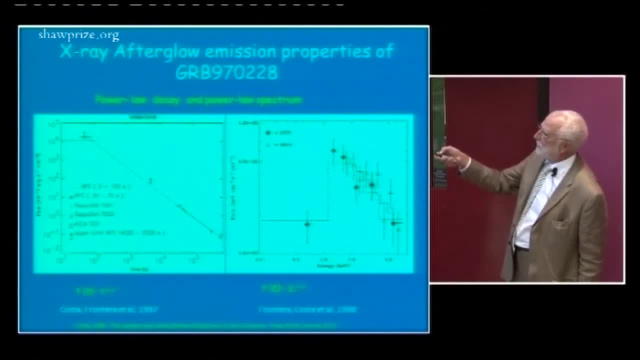 this is the prompt burst. This is where the burst disappears in Y field camera, And these are the points measured with X-ray telescope. Then we point again after two days. Here there is also a pointing of our Japanese colleague with ASCA satellite. 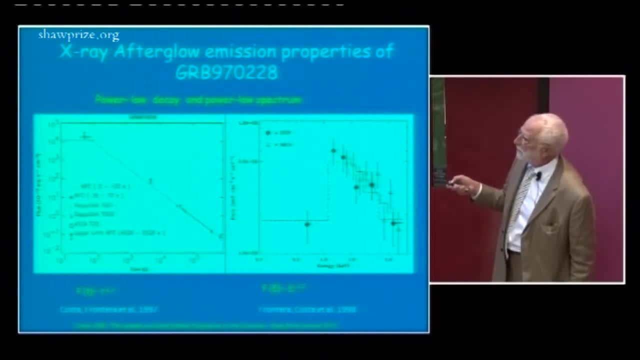 And eventually there is a pointing with the German satellite ROSAT, which is not yet here. So everything seems to decay following a power law. And also a power law is the energy spectrum. This is important because a power law is not a hot ball of gas cooling. 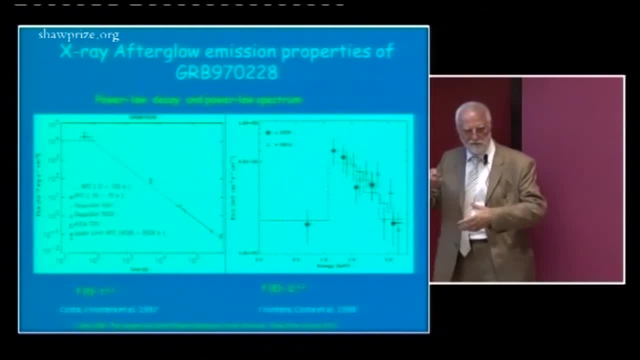 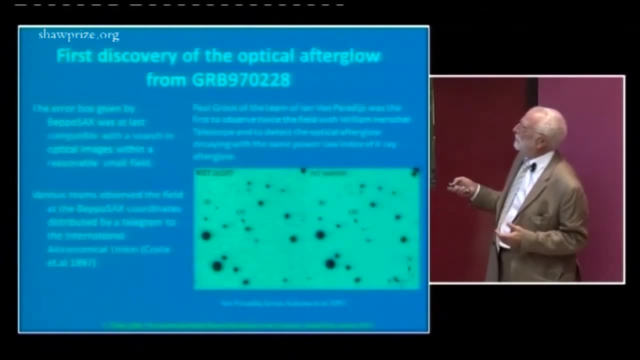 and is not a radioactive decay Power ball means something dynamically connected, Typically an explosion, And on the position given the Bepo-Sachs, that now was around one arc minute precision, many groups pointed their telescopes, And the first, what was important, is that 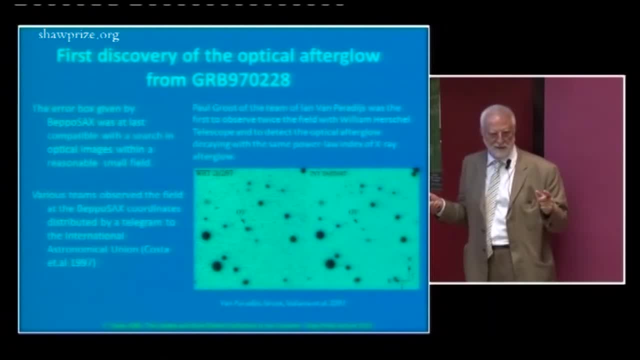 the source associated was that faint that it was not, could not exist, was not comparable to any catalog. So what was needed was to have at least two images of the same field and find the source that had faded. And this is what did Jan van Paradijs. 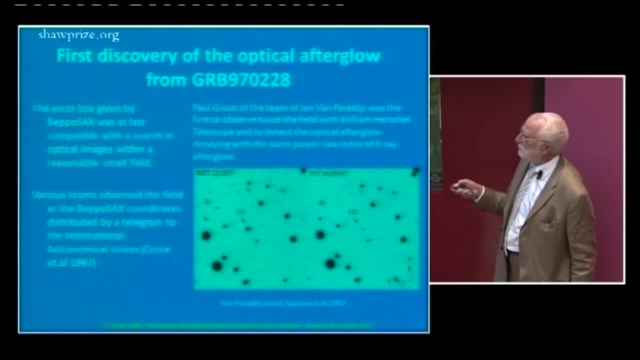 with his PhD student, Paul Groth. They had, they were the first to have two images. One was nine, eight days, I think, after the burst and one was immediately after the burst. So this was the optical transient. With this you go from. 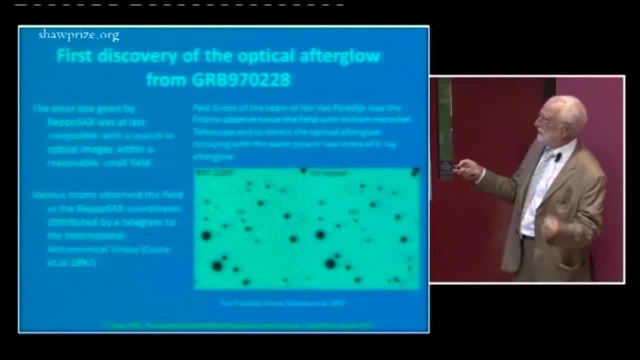 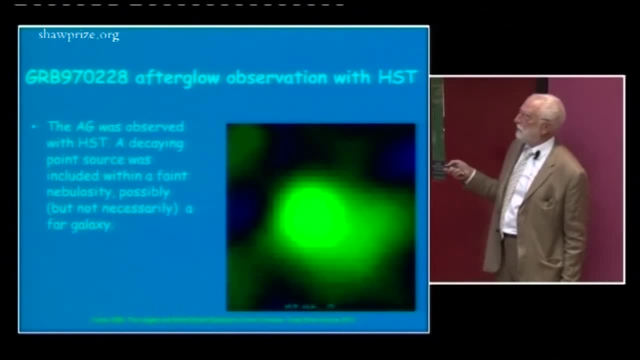 the one arc minute given by Bepo-Sachs to arrive to one arc second, which is the resolution of optical telescope. The source was also pointed with Hubble. With that you go better than arc second And most of all, there is a clear evidence. 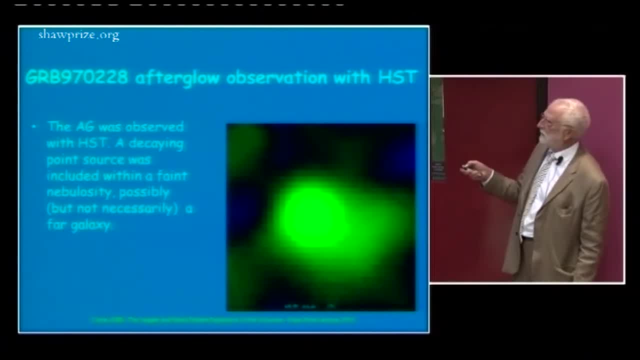 of a nebulosity. So this is the point source, the one which is fading, But since the optical telescopes are more and more sensitive, you can still detect it, Even if it fades to very low level. there is a small nebulosity. 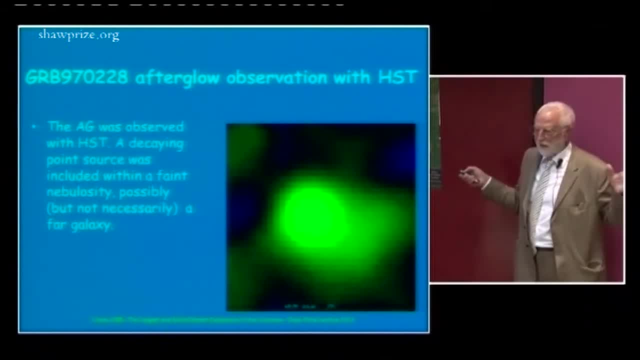 So likely a galaxy Like a galaxy, but of course you have many nebulae in the sky, So it can still be something galactic. And still the supporters of galactic hypothesis say: OK, clear, that's a neutron star. 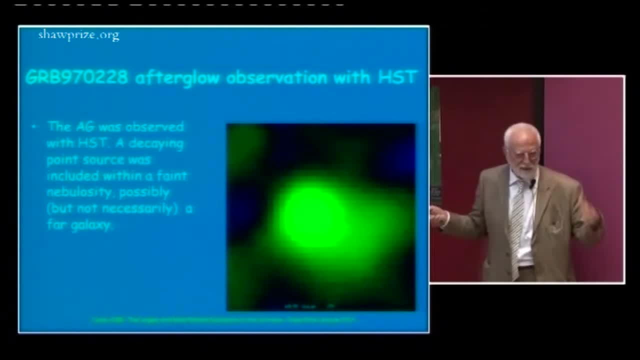 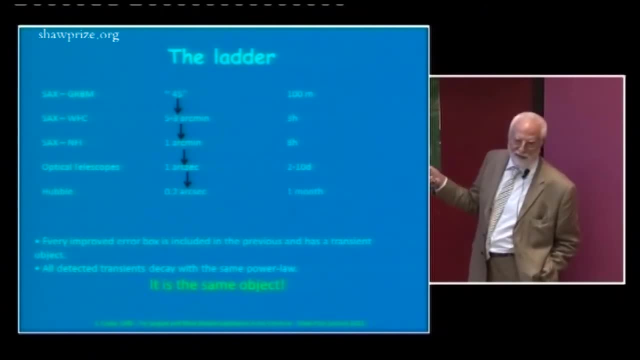 and that's the remnant of the nebula following the explosion. So I want to just remind what we call the ladder. I mean that just by pointing the direction of the map we would never find, because the source was extremely faint And in a field of one arc minute. 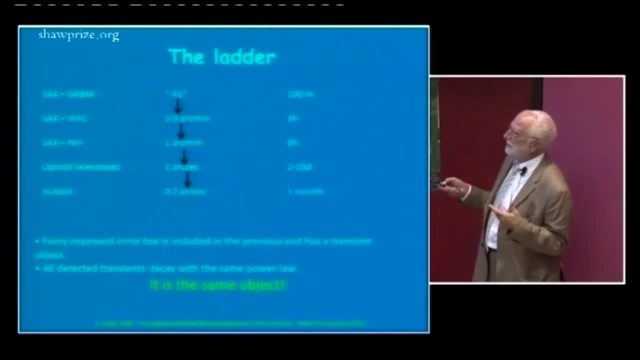 you have many galaxies You never associate. So what was needed is to follow the same source, changing. First, you detect with the gamma burst monitor and you have this data available after three hours. Then you can arrive. You just know that it is on that side. 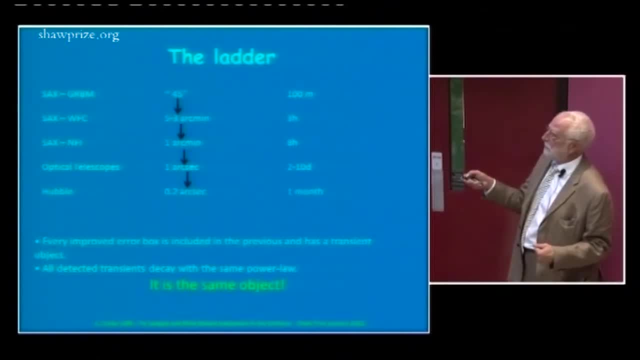 of the satellite With wide field cameras. five arc minutes in the beginning. Eventually we arrive to three. With the narrow field, one arc minute, But this takes eight hours. With the optical telescope, you arrive at one arc second With Hubble. 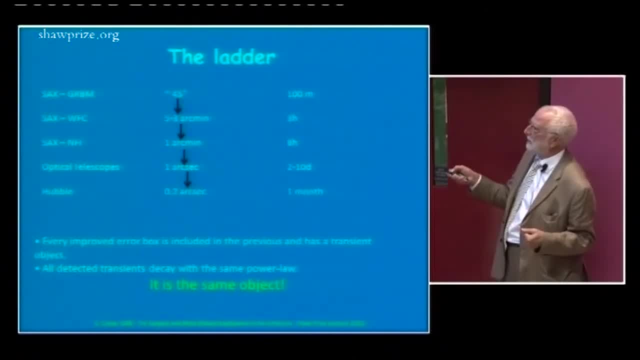 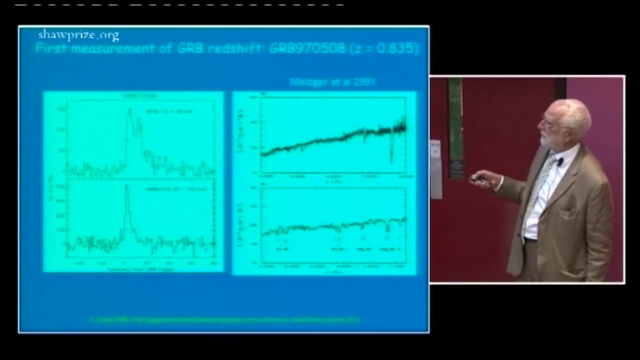 it goes better than one arc second, But typically they don't point So through this ladder we know that this was the same object. The next step is two months after, when we detect another gamma burst with gamma burst monitor. we detect with. 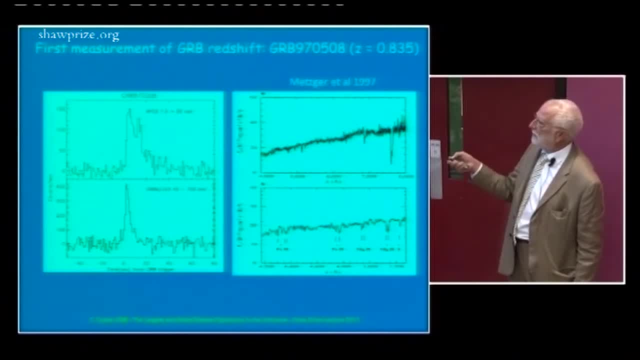 the wide field camera And the Keck telescope- that was the largest in the world at that time- was pointed And they took a spectrum and found the clear evidence. It's not clear at all to me, but for a spectroscopist 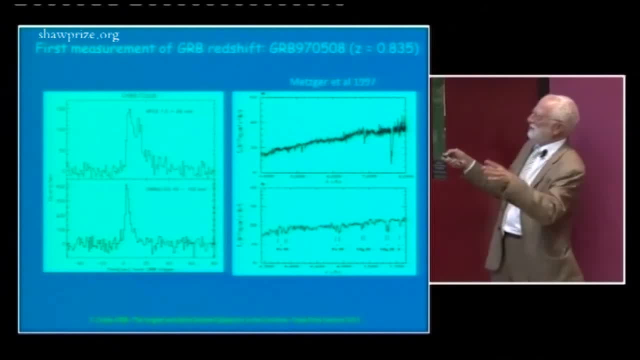 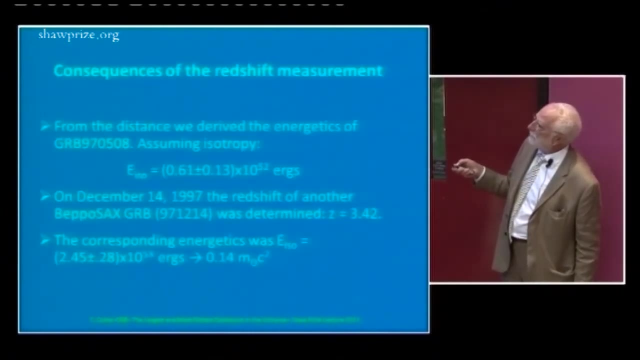 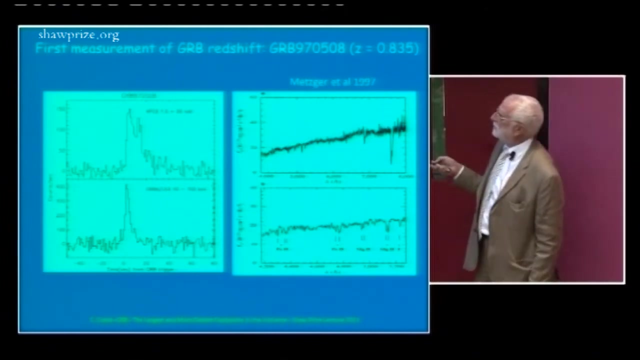 for a trainer. it's very clear. This is a typical spectrum of a galaxy with absorption lines And these absorption lines are shifted. This means that the source- I think I'm missing that this source- is shifted to the red of about 0.8.. 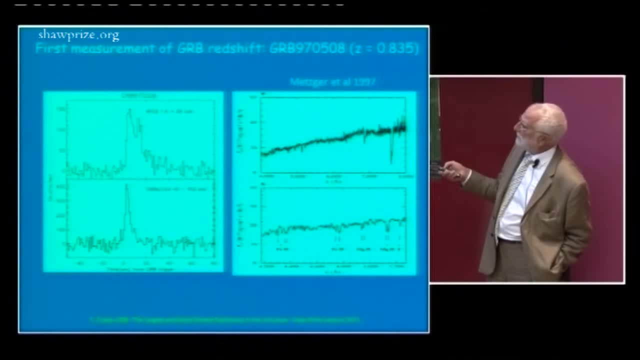 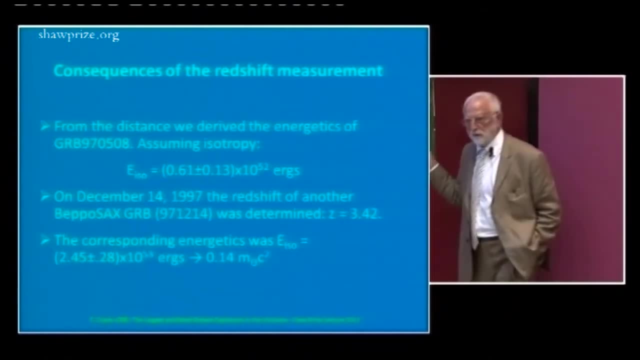 And this is the clear demonstration that the gamma bursts are extra-galactic and they come from very far away. This is around five, six billions of light years distance. This immediately puts a limit to the energy If the emission is isotropic. 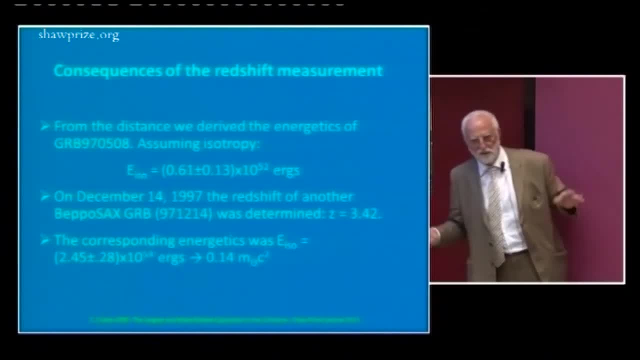 of course, we can also measure what comes in our direct, But in the assumption that it's isotropic. this means 0.610 to the 5.2 Ergs And this means that this is a significant fraction, is about a significant fraction. 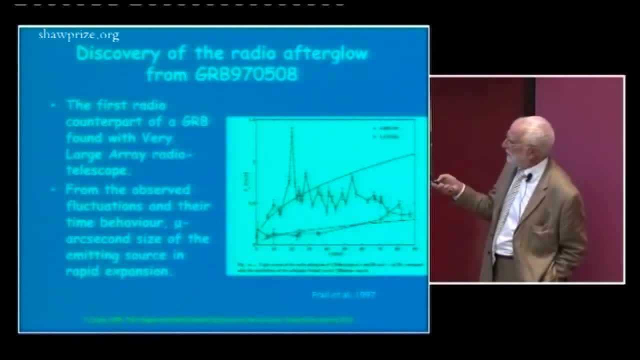 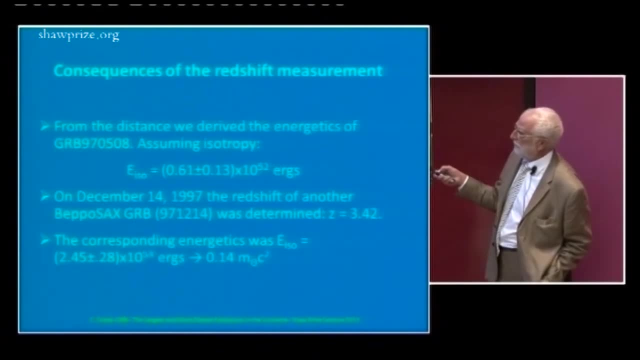 of solar mass. The same year in December we detected another burst that had a redshift of 3.4,- very far. The corresponding energy was 0.14 times a solar mass converter into energy of photons in about 10 seconds. 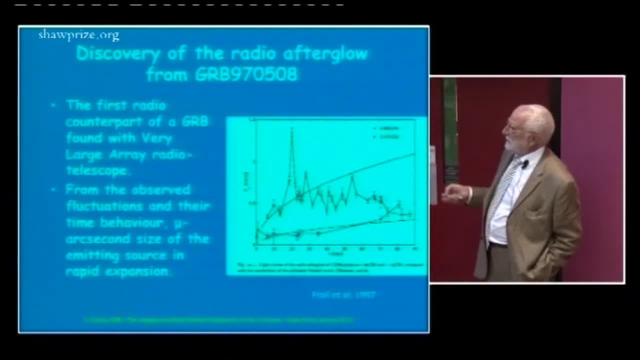 So this fixed the scale of the energy. There was another very important result on that burst of May 8, 1997, that also the radio afterglow was detected. And this was very important because this afterglow shows a very strange behavior. And this is well known to radio astronomers. Its name is scintillation. It's something that they find in pulsars. I mean, if the source is very, very small, the clouds of ionized matter in between the direction produce this effect. 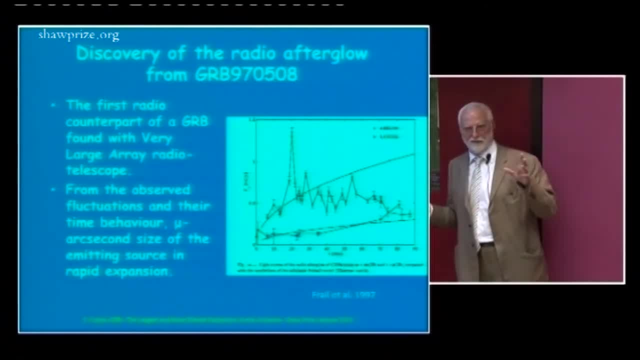 And this is exactly the same for which we see stars that are blinking, While the planets have a steady light. our light has not the resolving power sufficient to distinguish a planet from a star, because both are below our resolving power, But the scintillation 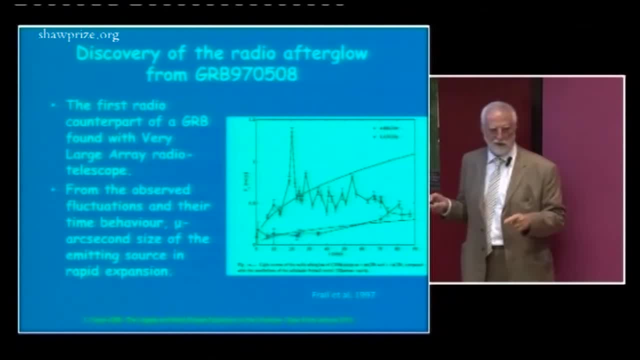 of the atmosphere gives us the information that the planet is above is above, let's say, 10 arc seconds, which is the Now radio astronomers have derived very well the scale of scintillation from pulsars which are almost point-like, so that's something. 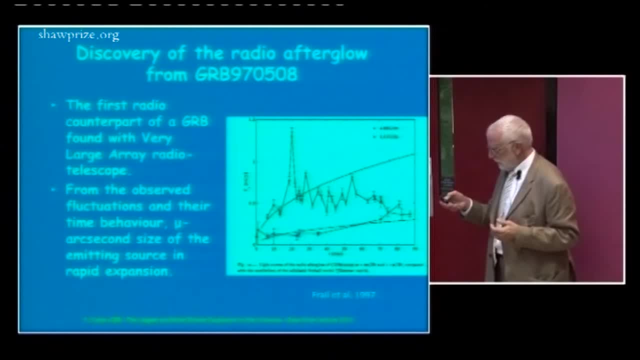 like four or five micro-arc seconds. So what you know is that this source is expanding because after two months, after two months, scintillation is stopped. This is when the thing arrives to an angular dimension superior to the typical angular scale of scintillation. 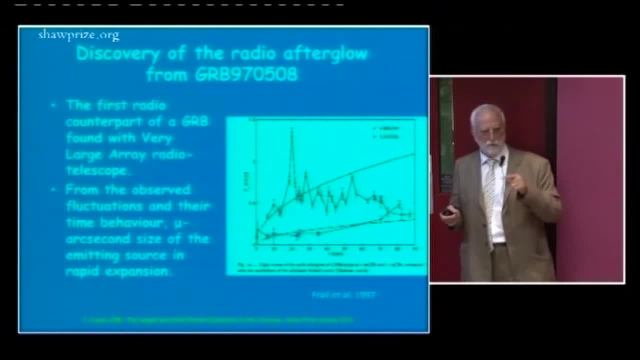 Now with this you can also compute which is the angular expansion of the source. You can derive the velocity of expansion of the source And the velocity came out to be 2c. Let's say this is expanding at an apparent velocity. 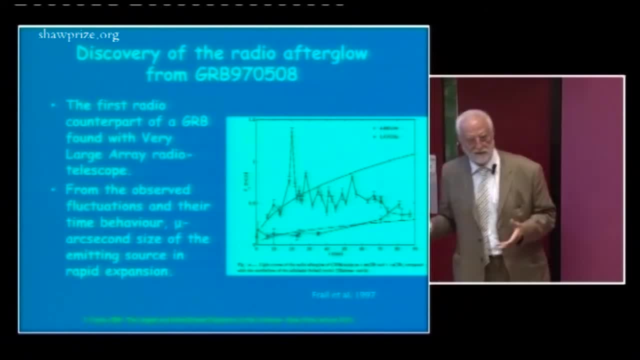 superior to the velocity of light, Which is something that, in extra-galactic astronomy, is not unusual and, of course, has nothing to do with the violation of special relativity. It's an apparent phenomenon due to the fact that the source is moving toward the observer. 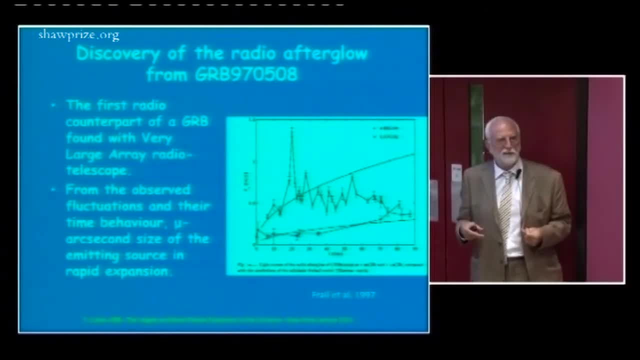 with the velocity close to the velocity of the light, So that while the light is arriving, the source is following very nearly and when it emits new photons we have the impression that they are going to the side effects, that they are moving faster than light. 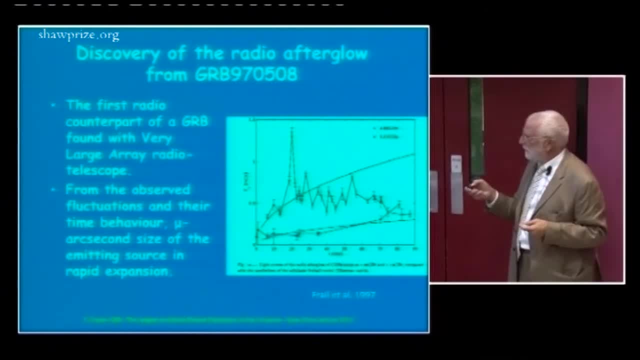 But they are not. But this for sure tells us that this thing is expanding at velocity close to the velocity of light. So this definitely is an explosion. It's not a supernova. A supernova is expanding a few thousand kilometers per second. 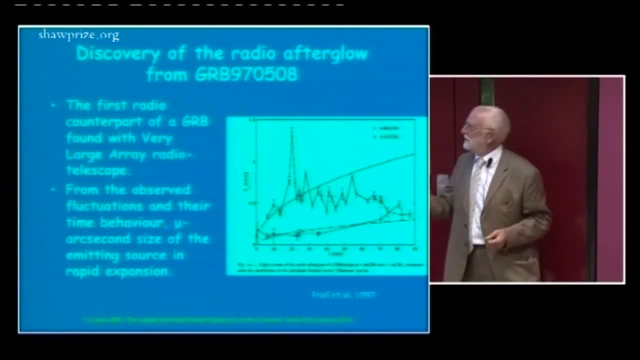 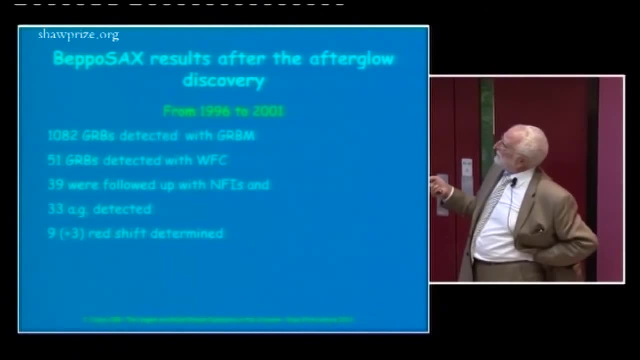 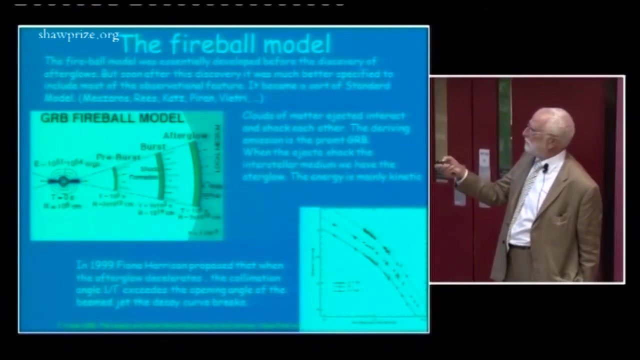 which is a lot, But you cannot see anything like this from a supernova. So let's say that this is basically what we did. Then we worked for four and a half more years. We detected 1,000 births with our birth monitor. 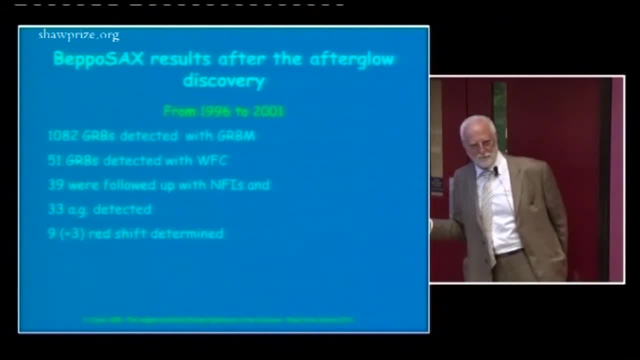 To be compared, let's say we detected 120 births per year, while Jerry Fishman detected 300. Of course ours was not a proper gamma birth monitor, So we detected 51,000 births associated in the Y-field camera. 39 were followed. 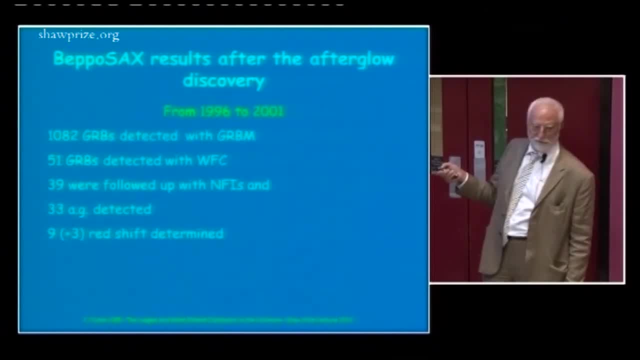 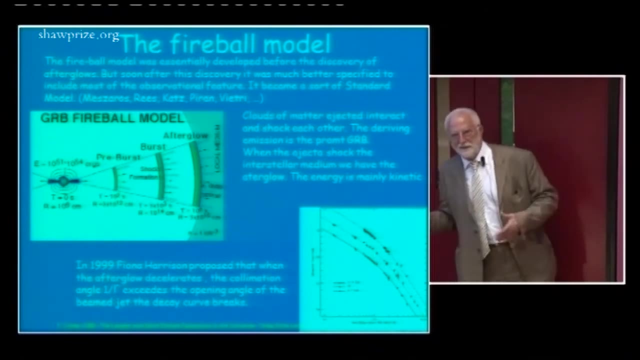 with narrow-field instruments We detected 33 afterglow On nine plus with less than three. we determined a redshift Now, soon after, immediately after theoreticians tried by using all the theories they had worked out before. 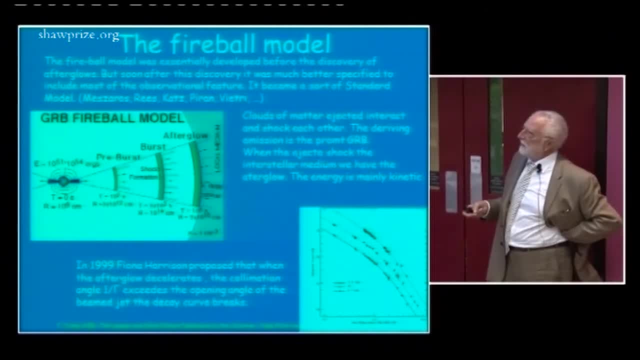 with the new data derived a model that became somehow a kind of orthodoxy, so that people proposing something different in conferences were not well. Let's say that that was somehow the mandatory model. I mean, you have an explosion From this explosion. 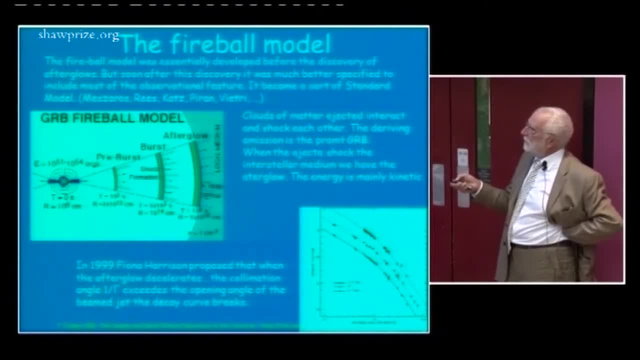 there is a jet and the explosion is ejecting some matter. This matter is ejected in the form of subsequent emission of mass at very high velocity, and this happens in the first seconds or in the first minutes, And then the shocks interact each other. I mean, they are ejected with different velocity so you have shocks and you emit energy And this should be the gamma burst itself. Then this ejected matter encounters the interstellar medium and transfers energy and heats this matter and this should be the afterglow. 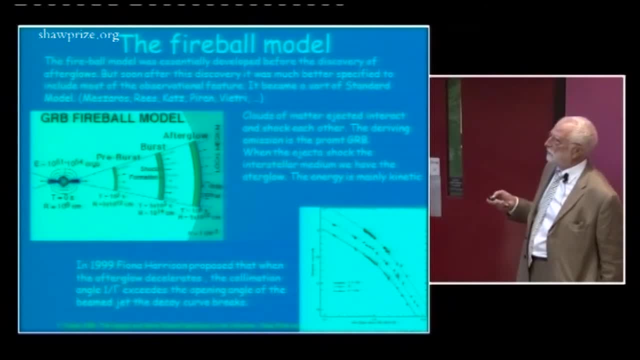 which also emits X-ray, radio and optical radiation. The mechanism of emission, the prevailing mechanism of emission, should be synchrotron, And the carrier of energy are a few protons, let's say baryons with high energy. 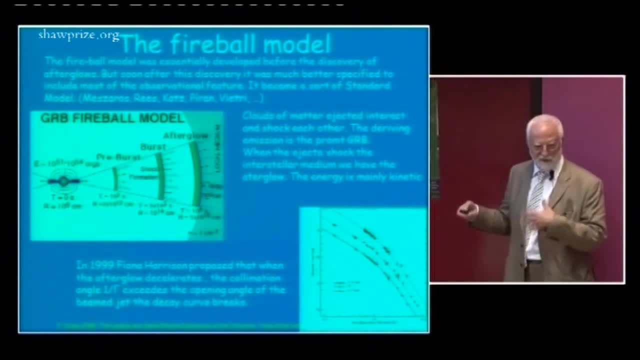 that are a small fraction of the total, but they carry almost all the energy, and the electrons are continuously accelerated and emitted by synchrotron because magnetic fields are onset or derived from before the elation. Another part of this vision is that gamma burst should be. 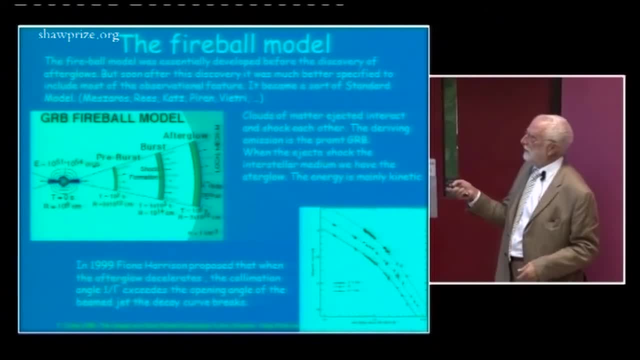 not isotropic and should have some opening jets with some opening angle, And one proof was that some of them show a break in their light curve. This break could be explained because, let's say, according to some relativistic effects, you only see if you have something moving. 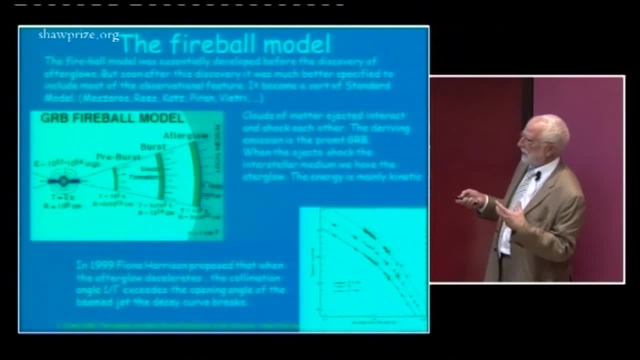 with a gamma Lorentz factor, you have like an effect of collimation. You see only those photons emitted in an angle below one divided by gamma. So, since gamma is decreasing, because this matter is lowing, when the gamma decrease and the angle is low, 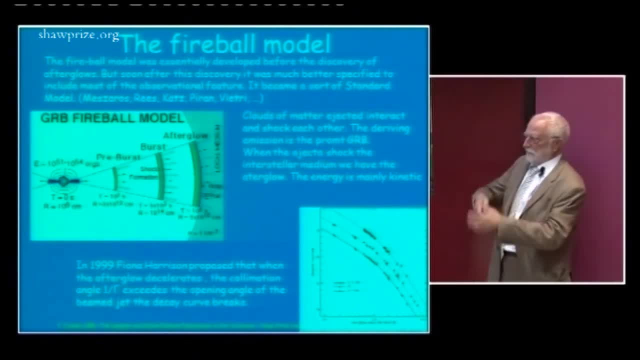 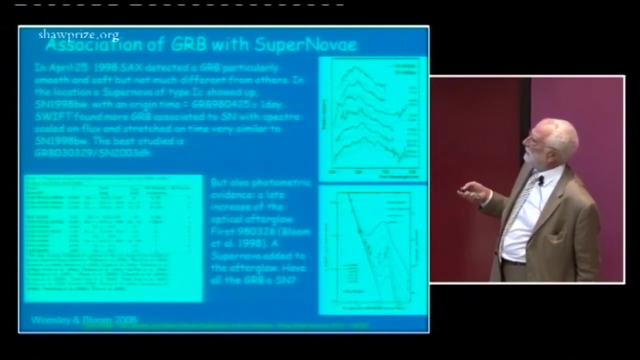 it is not large enough to include the jet, So you have no more matter feeding the process and you have a change of slope. This was the way to understand which would be the angle of the jet, And another important result was that in 1998,. we found a gamma burst that was associated to a supernova. It was apparently a normal gamma burst, but it was much nearer and much less energetic than all the others. Of course, we would never know if haven't we seen the afterglow and localized. And now there are more than 10 gamma bursts associated with the supernova, for instance, but we only got one with BepoSat. The others were found thanks to sweet satellites that arrived later. So there is this association, but only for very few bursts. 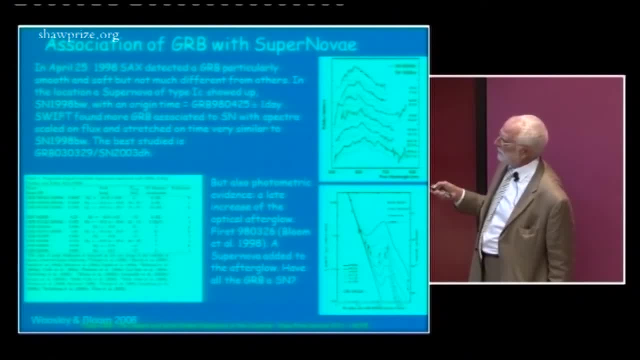 Or maybe not, because in some cases it has been seen that the afterglow light curve after maybe tens of days, one month with the powerful telescopes starts to rise again, And so if you imagine that in very far bursts you have something like: 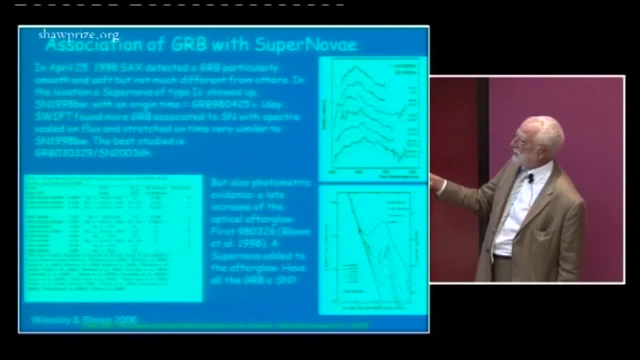 what has been seen in a nearby burst. this could be explained in the sense that all gamma bursts have an associated supernova And this can be detected, let's say, photometrically, even though there are not enough photos to take spectra. But for sure let's say that it's possible that all gamma bursts have an associated supernova and for sure most of supernova have not a gamma burst associated. After BepoSat we have two more missions dedicated to gamma bursts. HETI-2 and SWIFT. especially SWIFT is producing a huge number of results, I think more than 250 redshifts. What was important, what BepoSat missed, was to detect the shock burst. HETI-2 detected the first. let's say, SWIFT detected the first short burst and HETI-2 the first short burst with afterglow. So what came out is that short bursts are closer and less energetic than long bursts. Then the statistic has increased a lot. 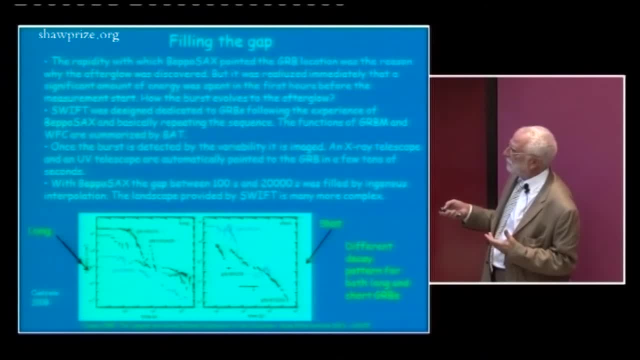 but the other point, let's say the major result of following satellites was the detection of short bursts. The other important result by SWIFT, because SWIFT was more or less conceived like BepoSat but the repointing was organized on board. 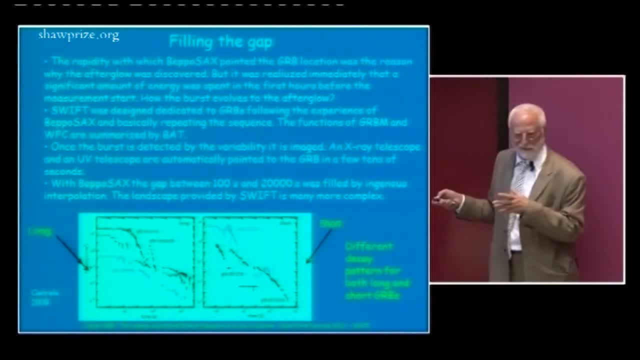 So while we arrived at maximum to repoint after six hours, they could repoint after one minute, even less in some cases, And so we knew now what happens between the gamma burst and the afterglow In the first tenth of a second. 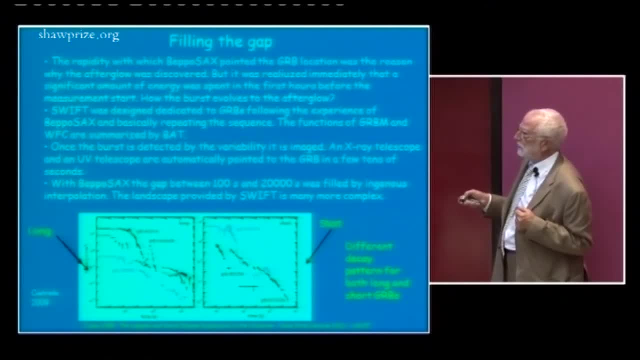 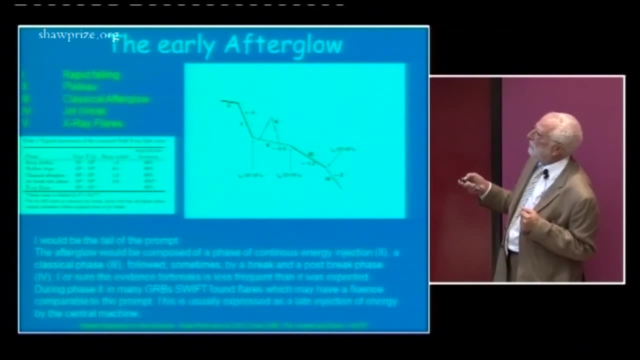 And this is a very complicated phenomenology. So there is now a kind of new paradigm And this is the main burst. how it decays. Here is the onset of the afterglow, when the matter is injecting energy in the afterglow. 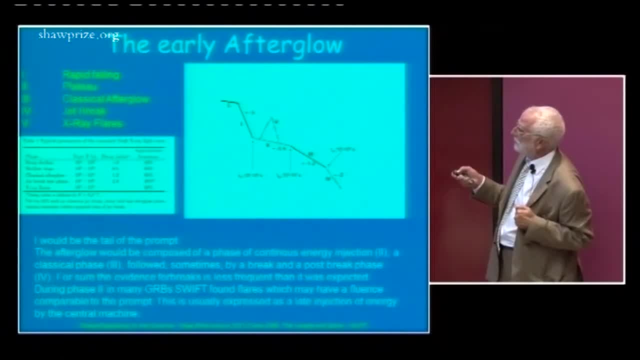 This is the standard afterglow- I mean that detected by BepoSat- And this is the afterglow after the break. What is important is that the numbers of bursts with the break are relatively a minority, while the time of BepoSat. 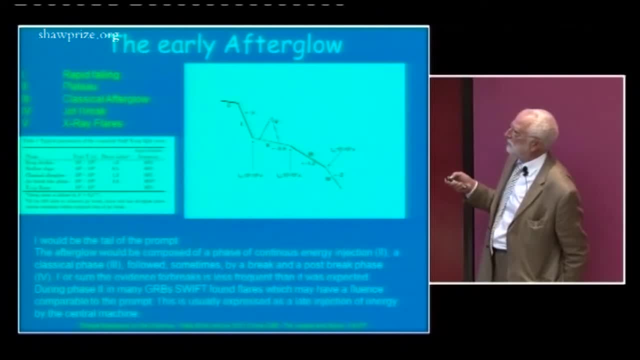 they seem to be a break almost for every gamma burst. All of this phenomenology is still mainly interpreted in terms of the fireball model. I mean internal shocks, external shocks, But there are also something very, very puzzling. I mean that in this phase, 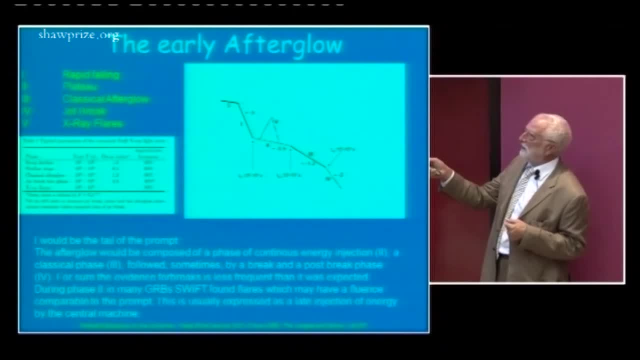 you have a re-bursting And since this re-bursting lasts more than the original gamma burst, sometimes there is an amount of energy comparable. This means that whoever is injecting energy and producing the shock is active still after tens of minutes. 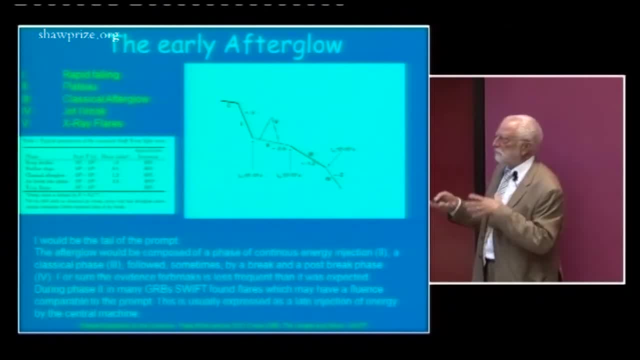 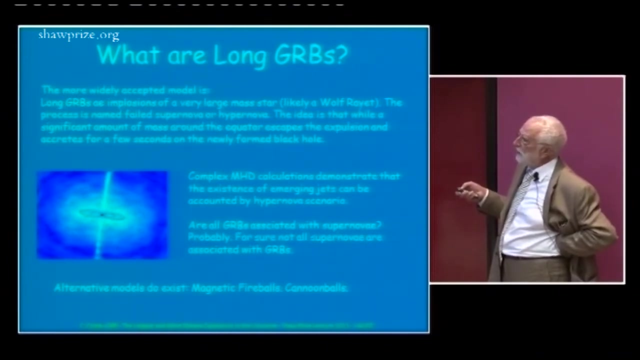 even more than that And this makes not that easy the explanation in terms of the conventional law. So there is a lot of work, proposal to discuss and to introduce new models. Now, what gamma bursts? what gamma bursts are? let's say that long gamma bursts. 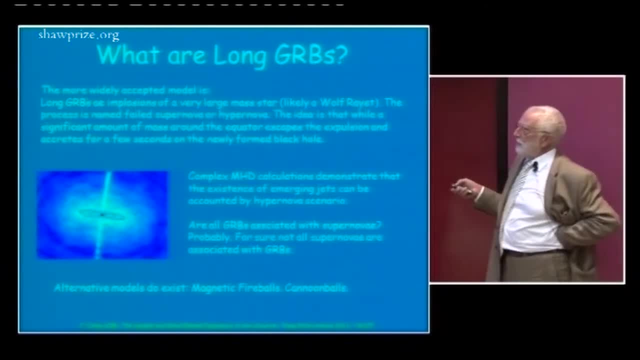 likely are the so-called hypernova or failed supernova. I mean that if the star has a very, very large mass- very, very large means 50 or more times the solar mass- when they collapse, there is not everything goes either in the black hole. or in the expelled remnant. But there is, for a very short time, a certain amount of matter of the order of fraction of solar mass that that circulates around the black hole and accretes in the black hole in few seconds or few tenths of second. 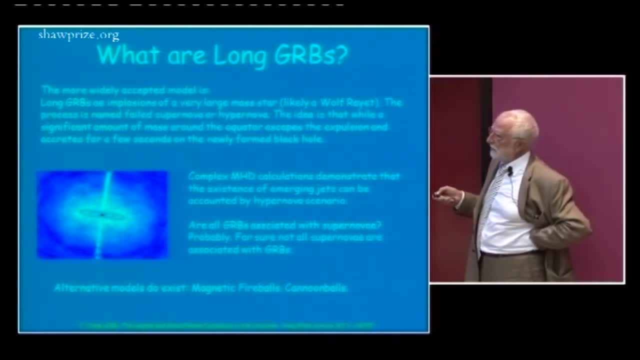 And this could be a very complex calculation of magneto-hydrodynamics, especially by and McFadden but many other teams that they can explain that in this case only a very narrow beams, very narrow jets, can emerge in the two polar directions. 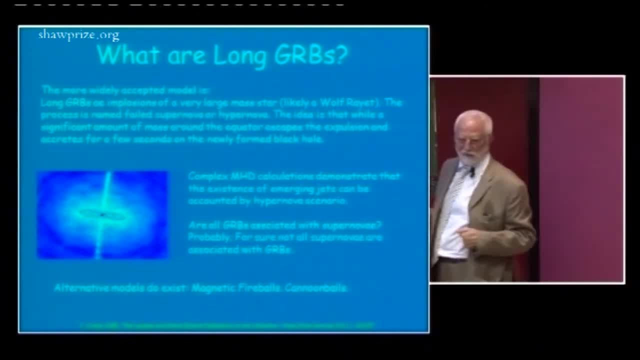 Now, if this jest is pointed toward us, we detect it as a gamma burst. Otherwise there would be in any case a supernova detected from all other directions, but the luminosity would be very, very, very, very lower, much, much lower. There are many people working on completely different models and, as far as short bursts are concerned, most of them have a redshift below 1.1 and typically 0.5, 0.4.. This means that they are closer and much less energetic. than long gamma bursts. The idea is that they could be two neutron stars that merge. There could also be the case of a neutron star and then black holes that merge. In this case, phenomenology would be slightly different, but also consistent with some sub-family. 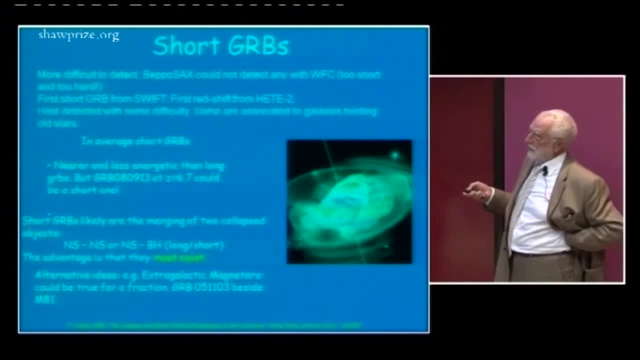 of the short bursts, And what is, of course, in favor of such a model is that this must exist because we know, for instance, that there are binary pulsars, And this pulsar first or later must arrive in the atmosphere. 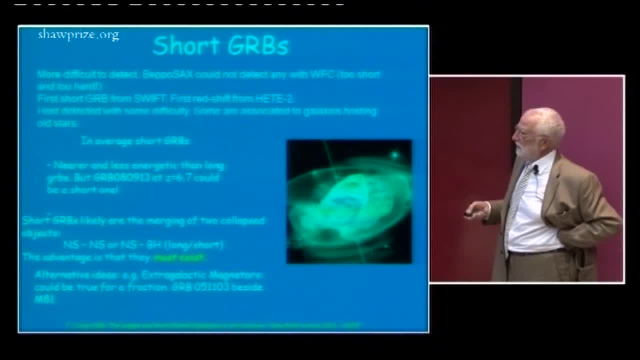 to the coalescence, So it is something that must exist. But there are of course other problems and there are many, many individual bursts that are very complicated and escape this kind of classification. For instance, one of these short bursts was close to a galaxy. 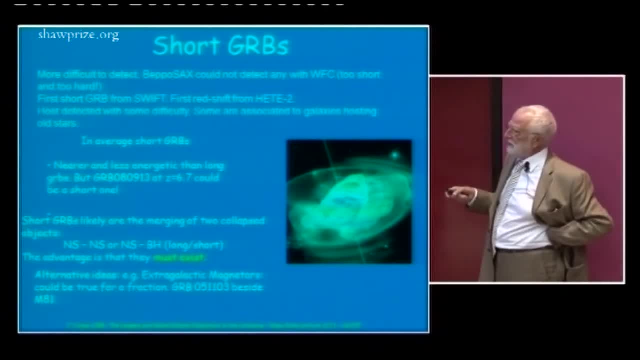 And since we know something which is an extreme phenomenon coming from neutron stars that are named magnet, if there are magnetic fields of the order of 10 to the 15, these are extremely bright, But in case they are still- they exist still 100 times brighter. 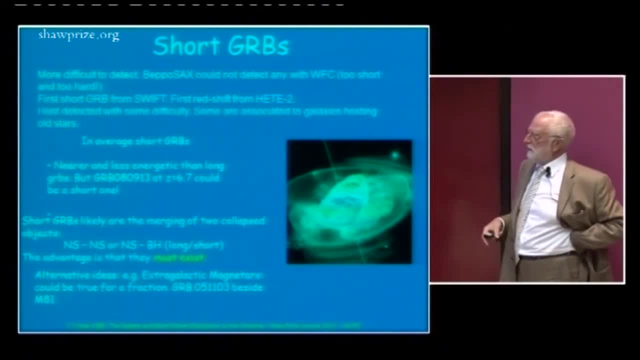 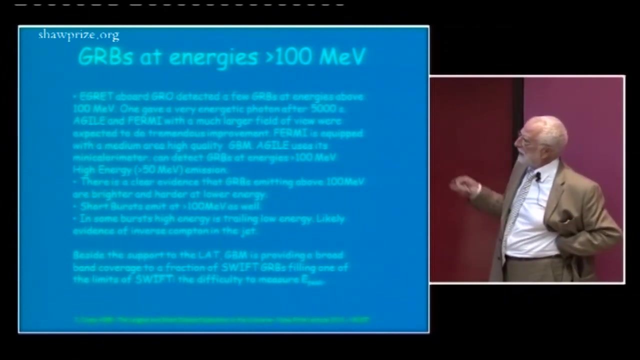 in nearby galaxies. they could explain a fraction of the short gamma belt. So actually possibly neutron stars have again a certain role, But this phenomenon is so rare that only exceptional events from other objects There has been an important contribution at higher energies. 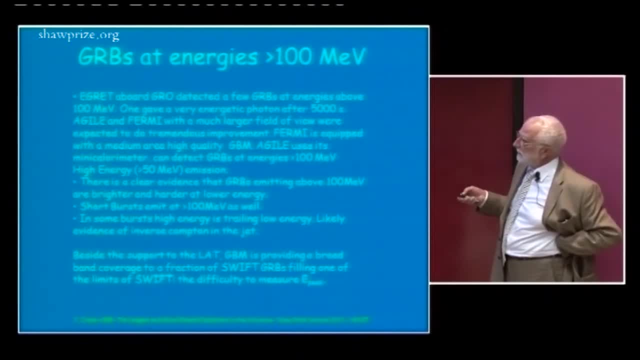 Satellites like Agile and Glaston- name them Fermi- have done a great job in detecting gamma belts above 100 MeV. The best surprise is that short and long in this energy band you cannot distinguish. They act more or less. 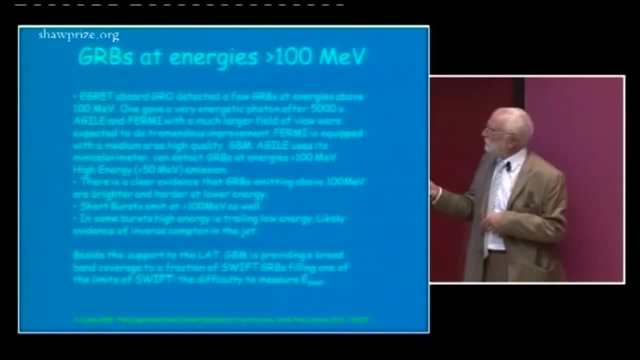 the same. Otherwise, it's clear that the phenomenology of high energy is not decoupled. More or less brighter and harder gamma belts are also emitting high energy. I'm not that impressed, But what is important is that, thanks to Fermi, 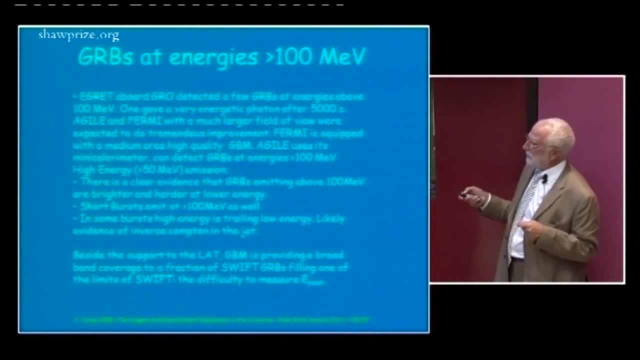 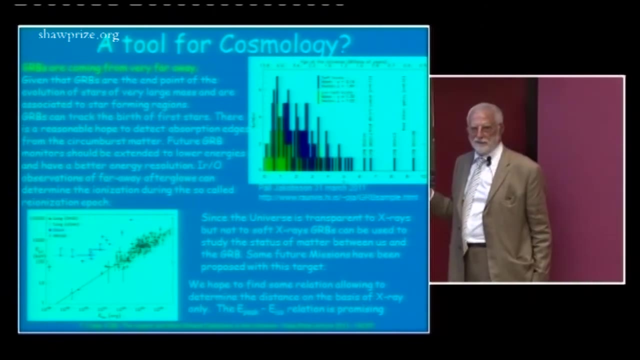 we have again a good gamma-burst monitor flying, built still by the group of Jerry Fishman, And this is good because, hoping to do cosmology by gamma-burst, We are trying to see whether we can do any use of these catalogs. 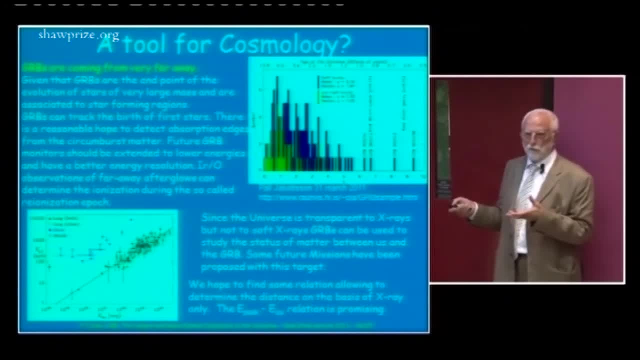 We have these thousands of gamma-bursts detected without knowing their range. So there is work to try whether we can derive the energy And one of these is done, started again by SACS data by our colleague- actually my student- Lorenzo Matti. 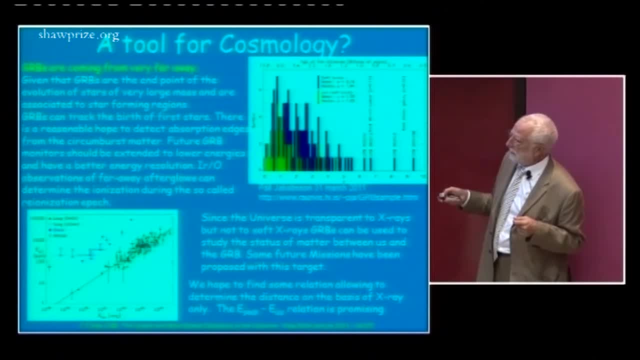 was he found a relationship between luminosity and energy at which the gamma-bursts peak. This is not yet having a standard candle, but can be a good ingredient. Some people is working on variability, and so could we find a way to derive the intrinsic luminosity. 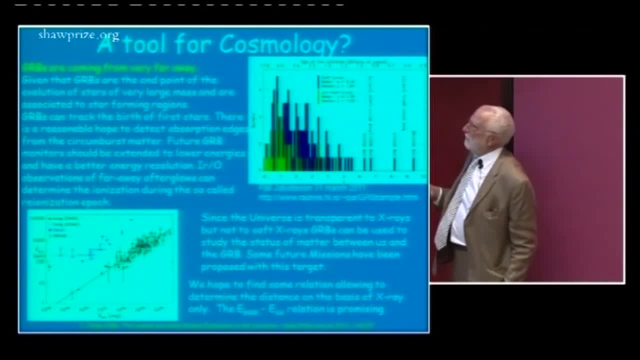 we could use these catalogs to make. So far, thanks to Swift, we have. these are the bars for which the redshift was derived. This is the redshift. This is the same converted into age of the universe. You see that we have. 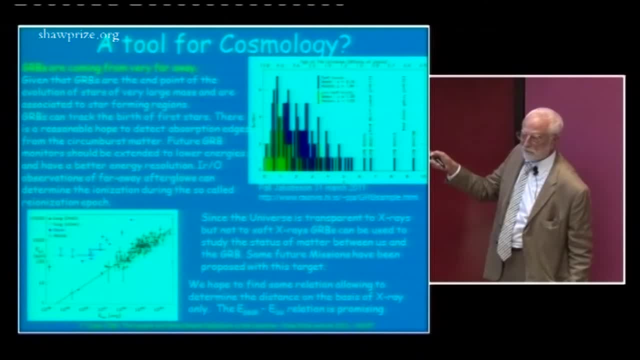 already four bars coming from the first billion of years of life of the universe. I mean that clearly these are in the so-called reionization era of the reionization era and when the first stars formed. Now did we start forming stars or forming? 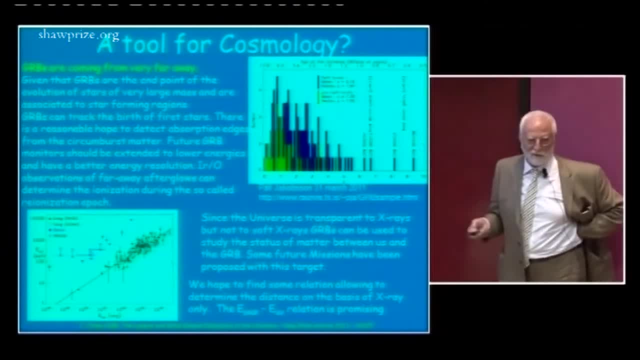 galaxies. Now we know that every galaxy has a black hole. When did these black holes were born? Of course, a gamma-burst is the birth of a black hole, So it's clearly I don't know exactly what, but a tool. 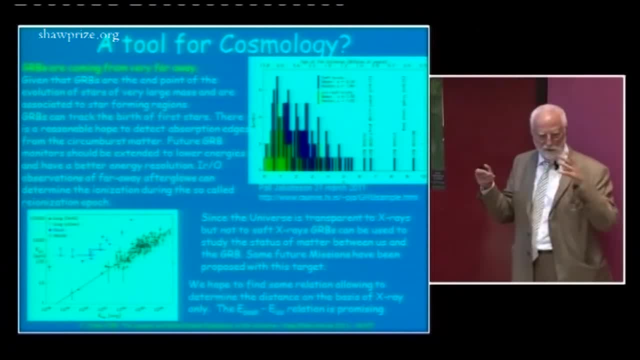 to do cosmology Also because we have the dark ages. we have the times when the dust not allows the light to arrive to us And X-rays and gamma-rays are. the universe is transparent for X-rays and gamma-rays, So for sure. 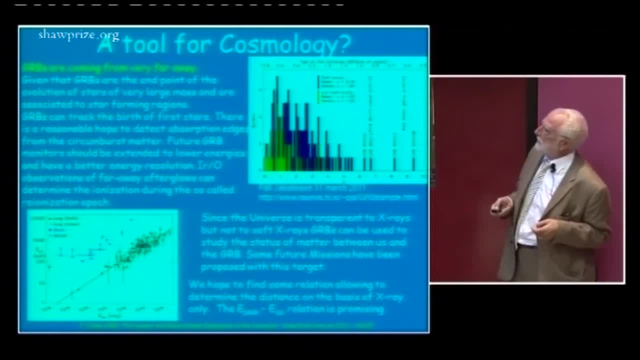 this is a tool that can be used in the future. So, in comparison with X-rays of optical and infrared afterglow, it seems that there is possibility to derive ionization, to have a direct proof, or the possibility to study through absorption so that 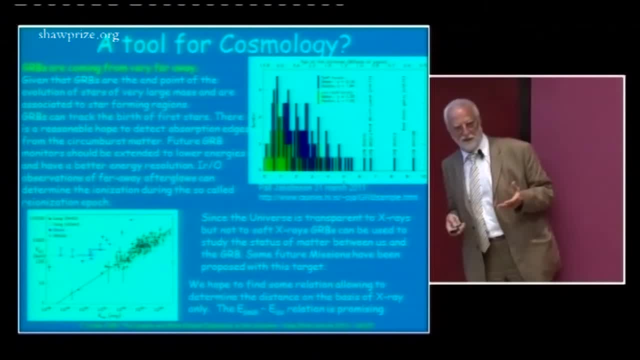 the intergalactic matter disappears And who knows? Everybody thinks that this is because it was heated to 10, to the 5. But this can be done by absorption of X-rays And this is important because this matter is organized with filaments. 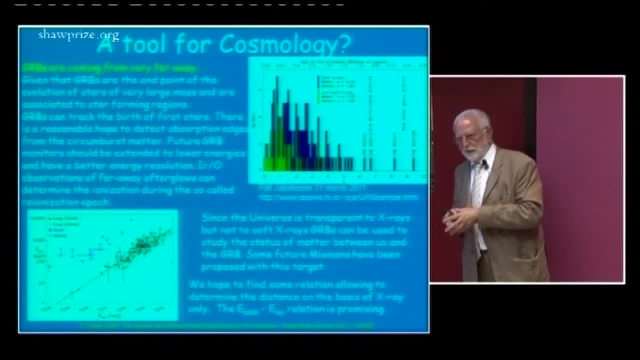 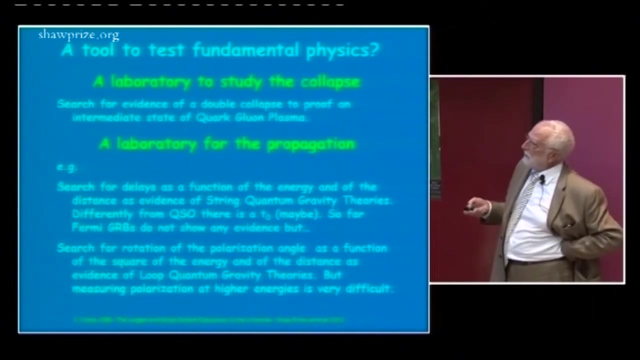 And these filaments are self-supported gravitation. So the idea is that these filaments are just showing, are just tracking filaments, organization of dark matter. So these are all points of high interest in terms of cosmology And gamma belts. 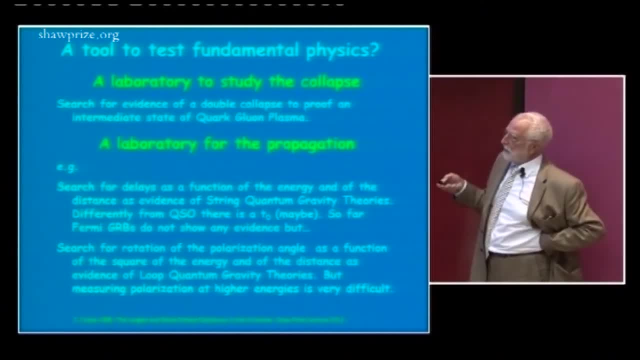 maybe will become that, And if you take those of the family of string quantum gravity, the velocity of light is slightly changing with energy, And this could be tested with gamma belts, Because gamma belts have started at the same time And this is all. 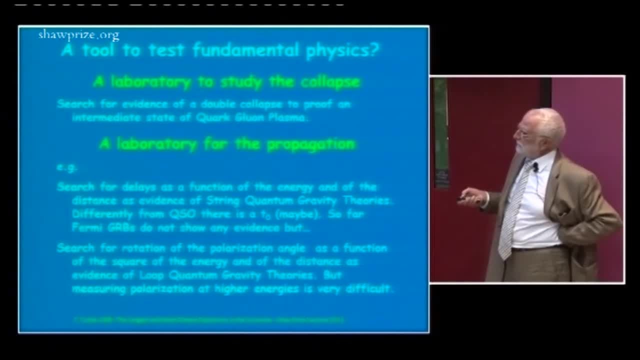 to be demonstrated. Another point is that the loop, quantum gravity theories and other big family predict that the universe should be birefringent And is that polarization should rotate only if you have some polarized source at a high distance. So this is.